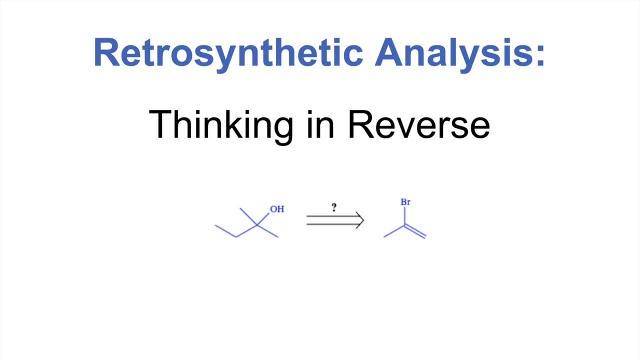 So today we're going to look at some newer ways of approaching synthesis problems. Synthesis can be a pretty tough thing for a lot of students. You might remember that all along I have taught you to think of synthesis problems, really looking at two things. You want to look at how the functional groups have 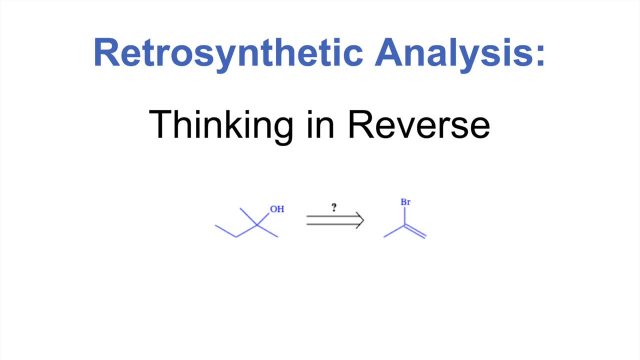 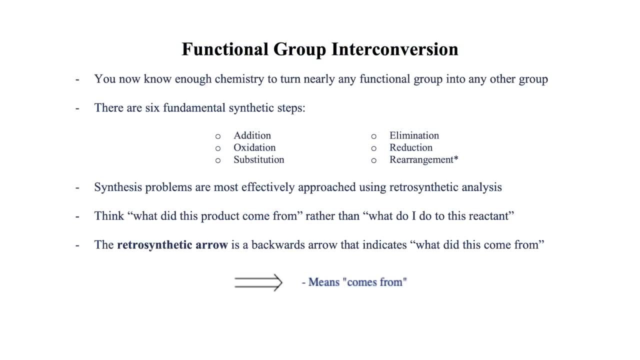 changed and how the carbon skeleton has changed. And when it comes to function group changes, believe it or not, you now know enough chemistry that you can turn practically any functional group into any other functional group. Now, when it comes to looking at reactions- organic reactions, there really only are six. 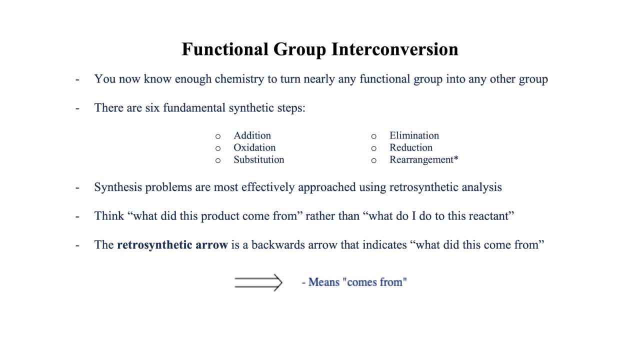 fundamental types of reactions. You have addition reactions, where you're literally adding a molecule across a pi bond. You have the reverse of that, which is elimination, in which you remove a molecule to form a new pi bond. You have oxidation, where normally you're increasing the number of bonds to 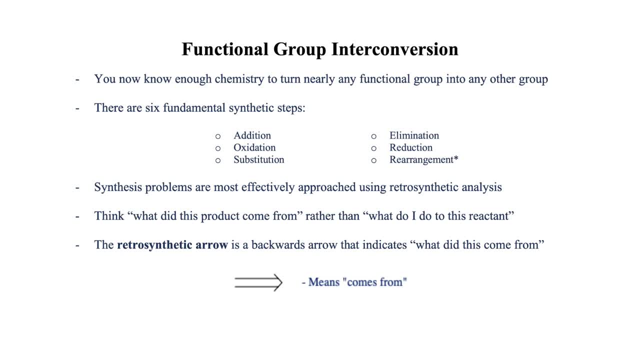 electronegative atoms, Again the reverse of that reduction, which is to decrease the number of atoms, of bonds to electronegative atoms. you have substitution: we're just swapping parts out. and then you have rearrangement, which is basically taking an existing molecule and somehow taking the parts and just scrambling them. 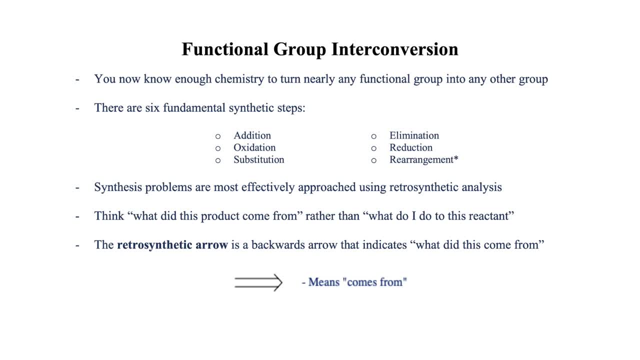 around, so they're connected differently. now we haven't talked a lot about rearrangements. we've actually talked mostly about rearrangements in the context of things like carbocation- rearrangements that are part of an existing reaction, not in a reaction in of itself. and when it comes to applying 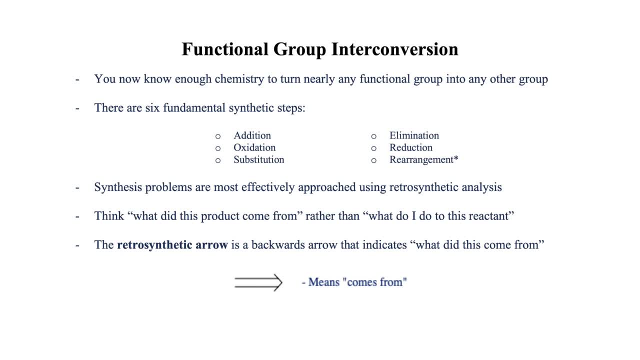 rearrangements to synthesis. that's really kind of beyond the scope of an introductory course like this. it can be really challenging to try to get rearrangements involved in synthesis problems. what we're going to do here is look at a new way of approaching synthesis, called retro synthetic. 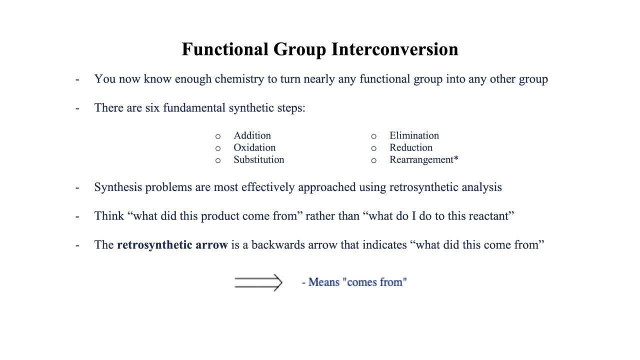 analysis. the way you look at this, it's kind of like thinking: what did this thing, this product, come from? rather than what did this product come from, rather than what did this product come from? well, what do I do to this reactant to make something else? it's thinking. 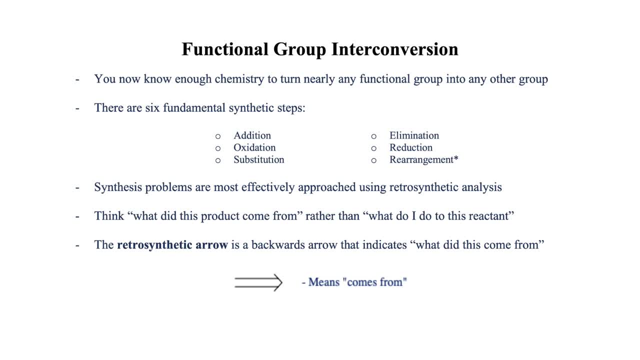 backwards and it has its own unique arrow, the retro synthetic arrow shown here. it's sort of a backwards arrow. I mean it looks forwards here, but it's it's interpreted in a backward sense. the way you want to read it is: this came from this. so what I'm going to do is I'm going to work you through a handful of 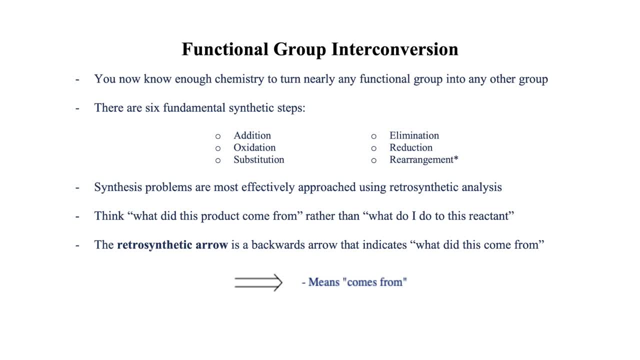 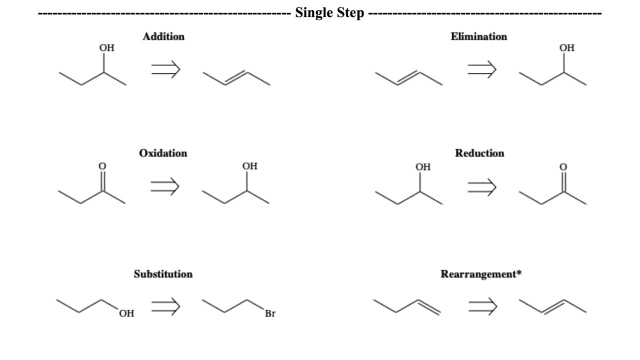 examples of some inter conversions of functional groups. we're going to start off by inter converting a handful of functional groups using one simple step and we're going to look at that retro, synthetically. so, looking at this, here we have one example of each of our six. 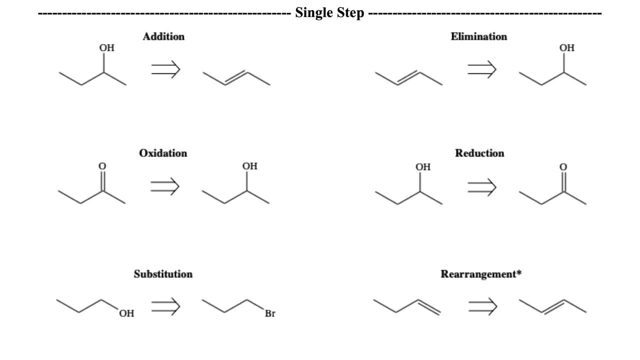 fundamental kinds of reactions. so look at this reaction here. it's a retro synthetic analysis. the way you read this is that this alcohol could have come from this alkene. okay, that's what I mean by it's backwards. we're not turning the alcohol into the alkene, we're saying the alcohol has come from a. 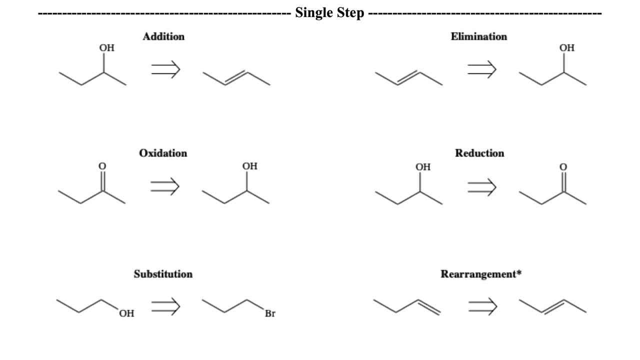 this alkene. if that alcohol came from that alkene, it would have to have come from that alkene via an addition reaction, specifically the addition of water. right, so we can go ahead and actually draw in in the forward sense what conditions would affect that reaction, for example, just water under. 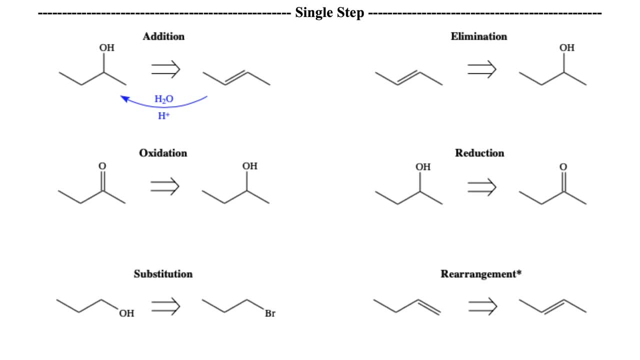 acidic conditions will do that reaction. so that's an example of how we look at things retro synthetically. you got to learn to read these, these retro synthetic arrows backwards, as if they're saying this is coming from this. look at an elimination. it's actually the reverse of 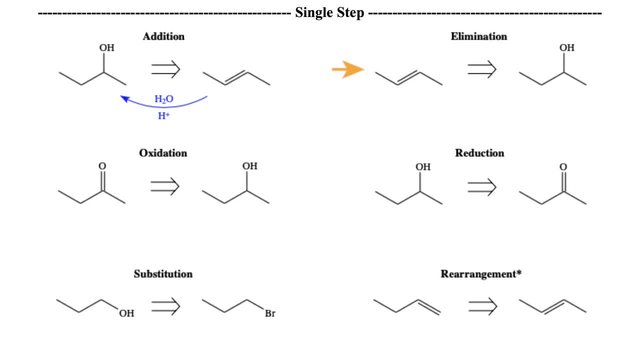 what I just showed you. again, this is saying that this alkene is coming from this alcohol, and if you want to make an alkene from an alcohol, that means you need to remove water. it's a, that's an elimination, a dehydration, specifically, and one way to do that is simply by heating it up with sulfuric acid. look at. 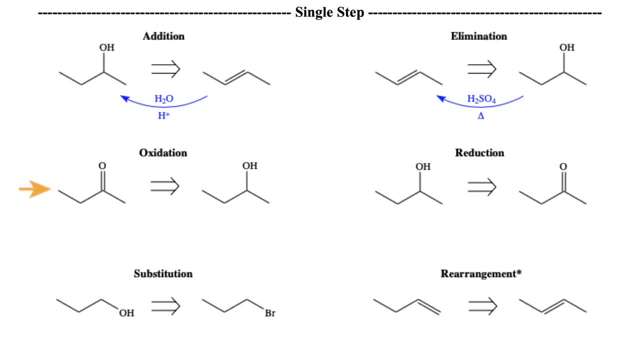 the next example. what we're saying here is that this ketone could have come from a, this alcohol, and in order to make this ketone from this alcohol, that would require an oxidation. you see how we've increased the number of bonds to electronegative oxygen, so a typical Jones oxidation, which suffice here. 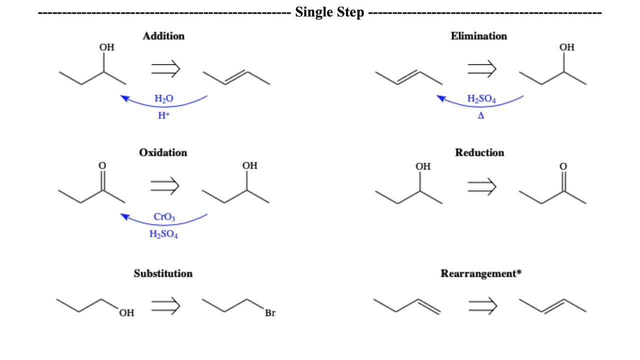 chromic acid right, chromium trioxide, sulfuric acid, for example, the next one we've got. this alcohol could have come from this ketone and to make an alcohol from a ketone that will require a reduction. so say, sodium borohydride, for example, useful for the 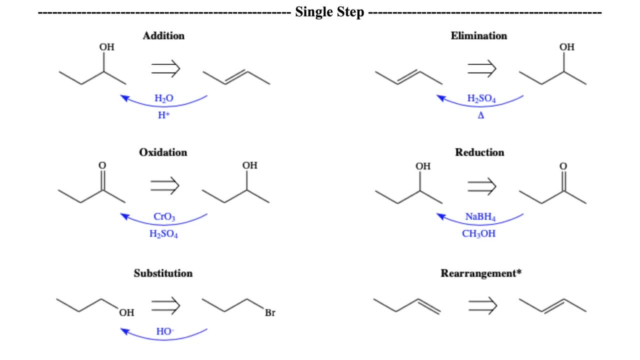 other radicals said for higher carbon emissions- glass fluoride, for example- this is the guess here in elephant 달 al- perceptions for a substitution of our. in one case we made an alcohol out of a situation where we have this protein eventually producing this purpose of alkene in methanol. next week got an. alcohol that could have come from an alko halide, and that's an example of a substitution. in order to make an alcohol out of an apple halide, we would need to do, you know, say, an SN2, a substitution here, hydroxide, would do the trick simply. 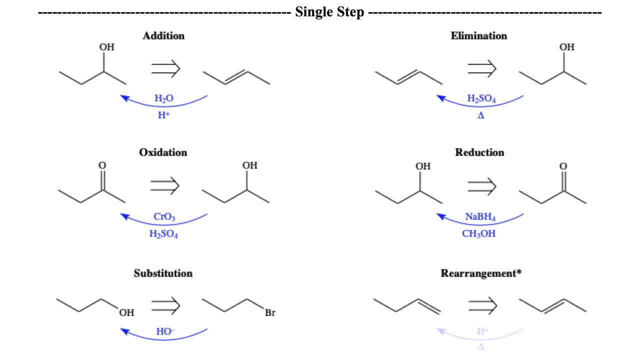 would be a rearrangement affected by, say, an acid, Heating it up with an acid, it could protonate and then deprotonate and go backwards and forwards. So these are some examples of how you can interconvert various functional groups via one-step process. right, And I'm 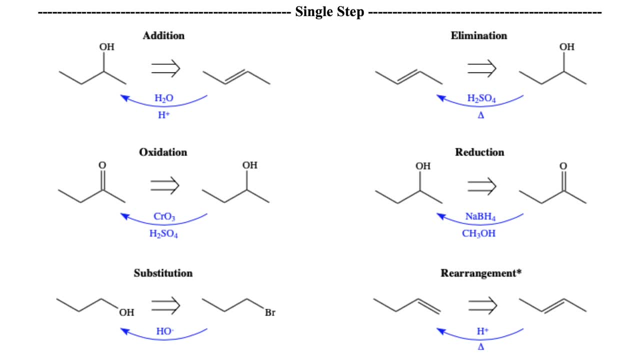 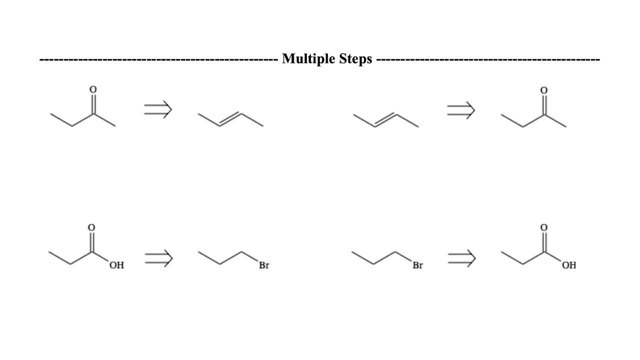 giving you an example, one of each type of fundamental reaction. Now, sometimes, when you need to interconvert various functional groups, it may take more than one step. So let's take a look at another example. Here I've got four examples that are going to require. 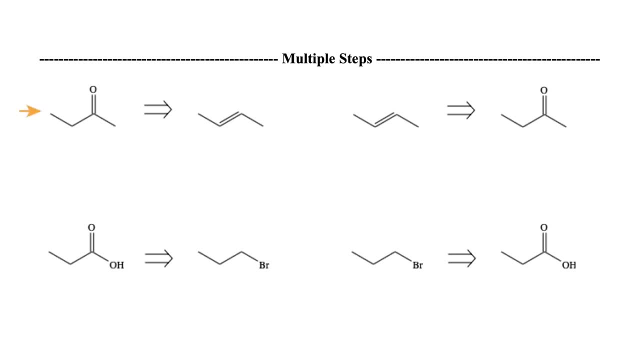 more than one reaction. So let's take a look at this one. This one is saying: this ketone could have come from this alkene. Now how do we make a ketone out of an alkene? There is no one single reaction that can do that. So to think retrosynthetically, what you want. 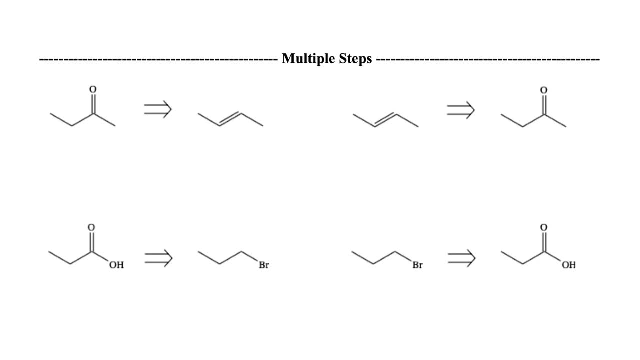 to do is say: well, what can I make a ketone out of? I know how to make a ketone out of, say, an alcohol, And then what you've done is created essentially a simpler, shorter, little retrosynthetic. 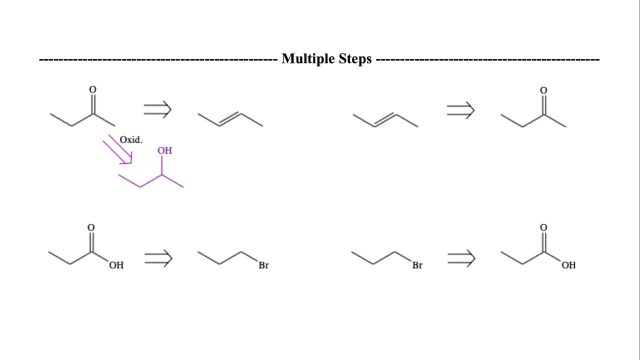 problem If you know that you can make an alcohol into a ketone. now we need to figure out how an alcohol could have come from an alkene. And, of course, an alcohol could come from an alkene through an addition, reaction, a hydration. 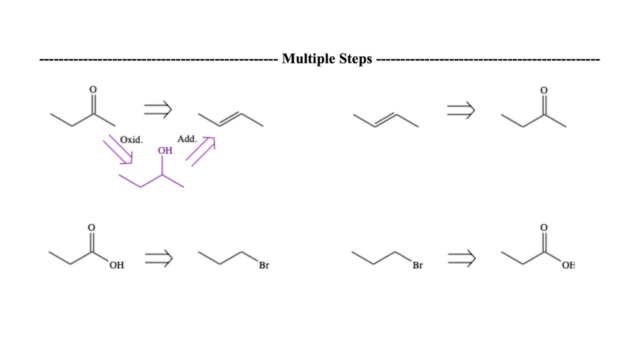 So we could go ahead, and that's our retrosynthetic analysis- And then, if we wanted to actually draw out the actual process, we could go ahead and fill in the conditions: Hydration with water onto the alkene to make the alkene. 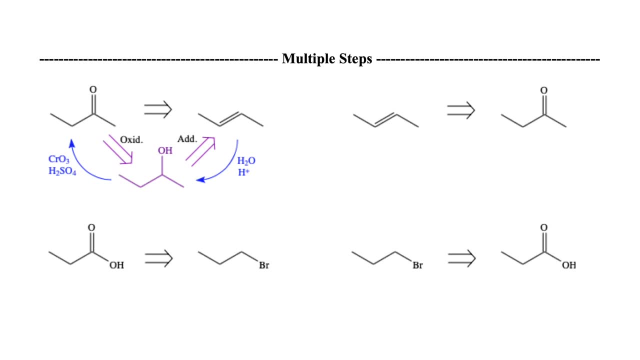 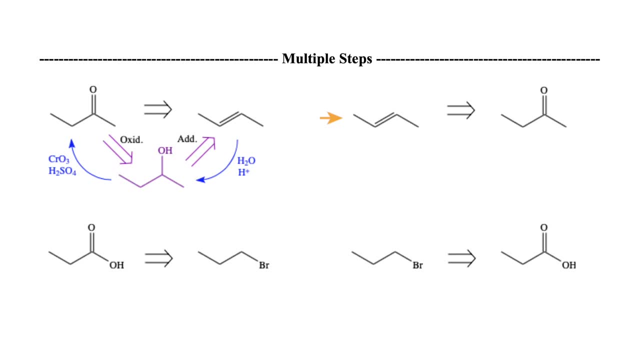 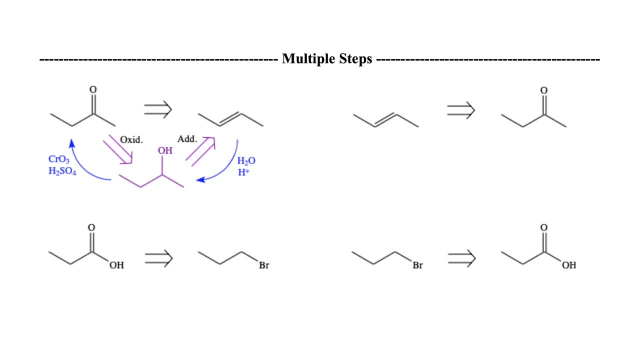 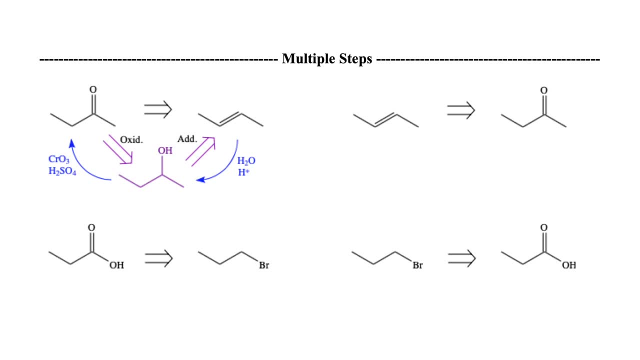 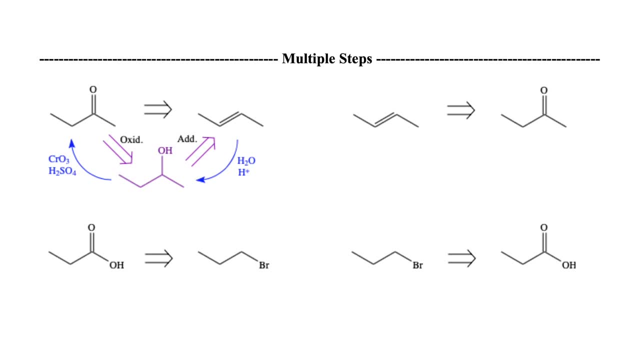 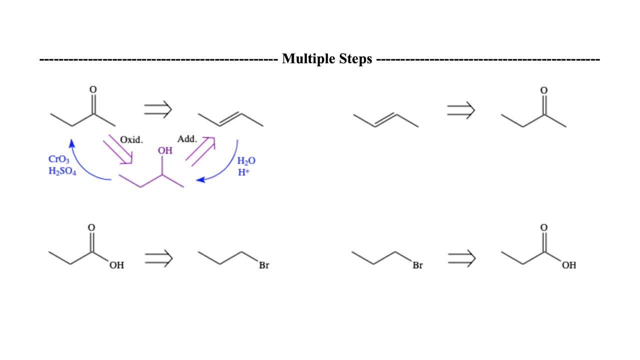 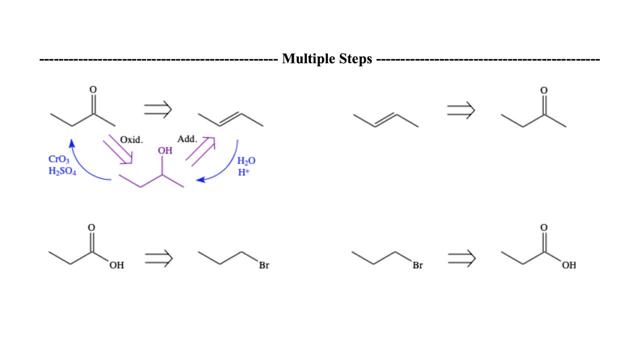 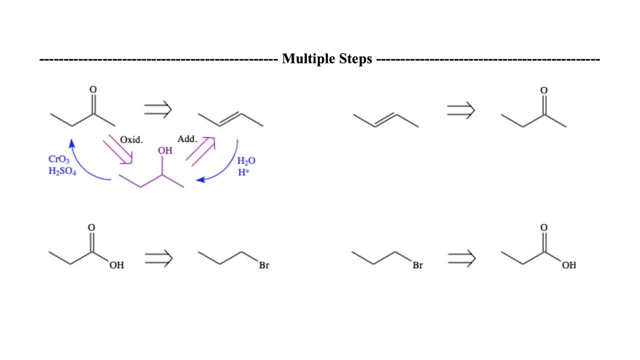 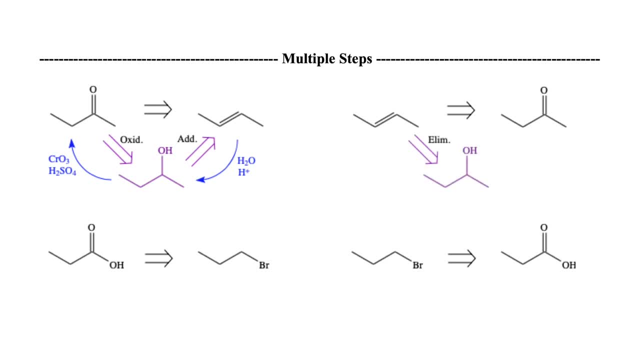 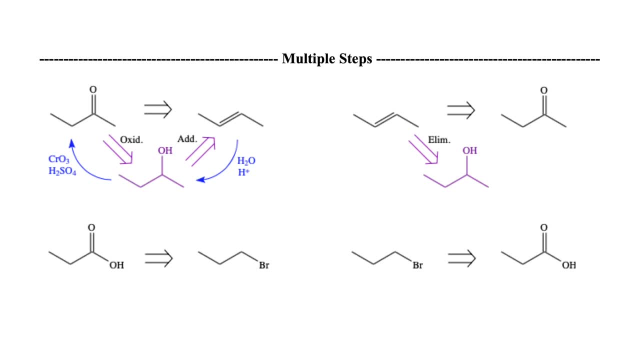 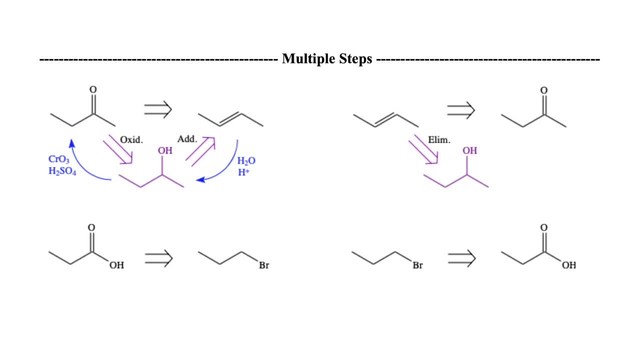 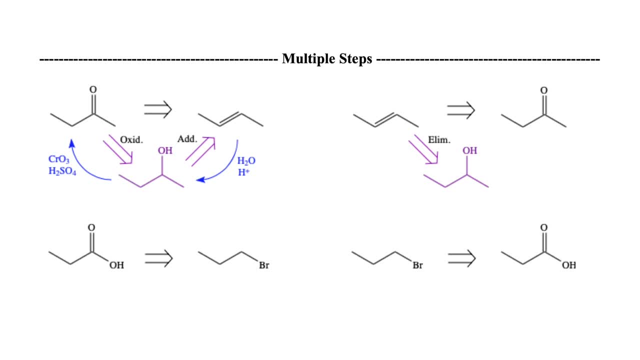 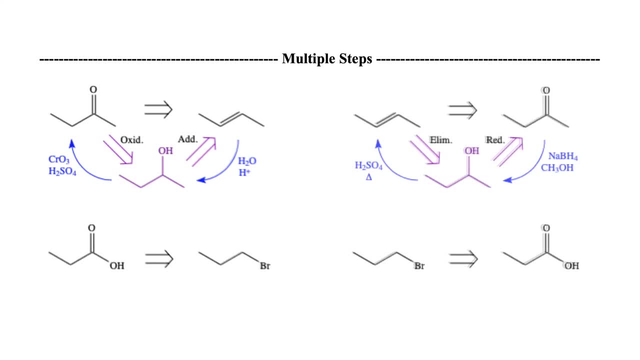 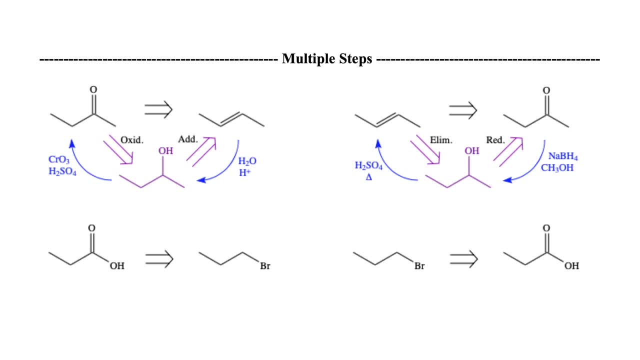 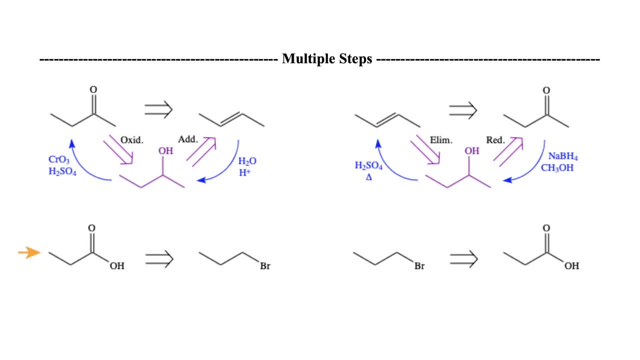 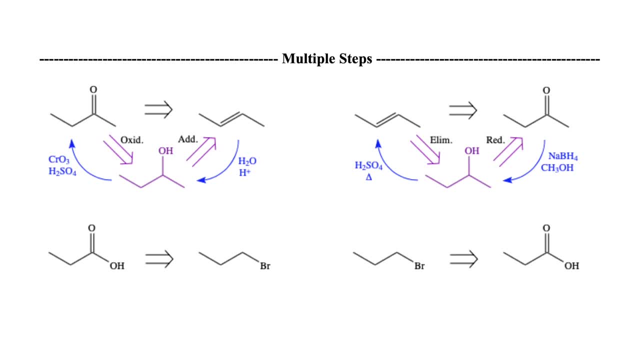 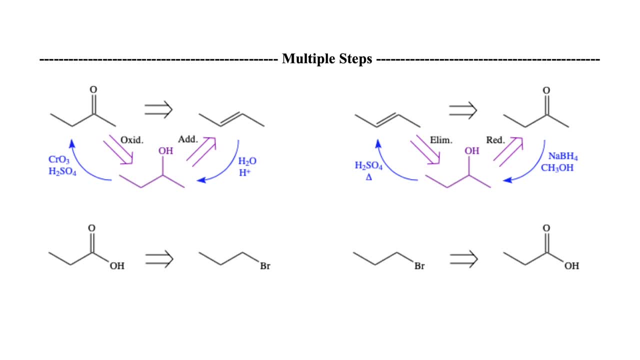 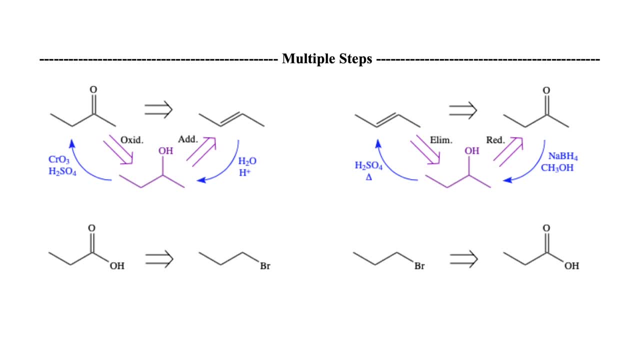 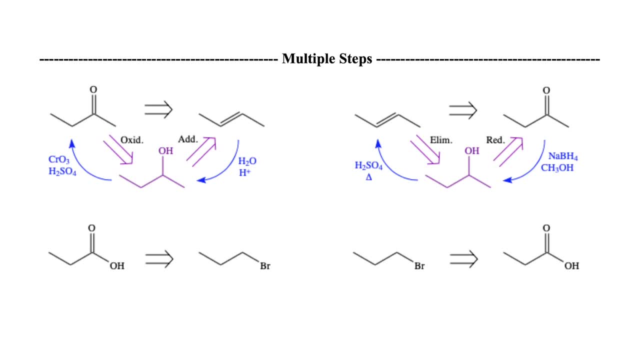 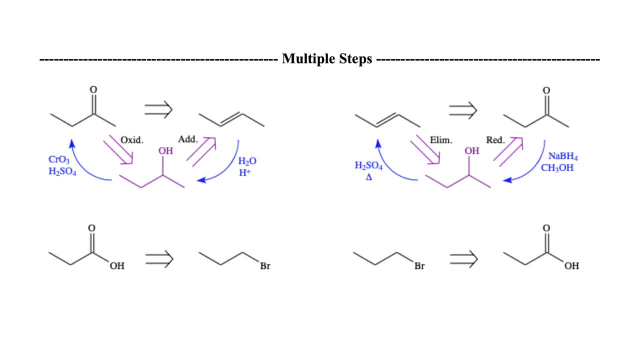 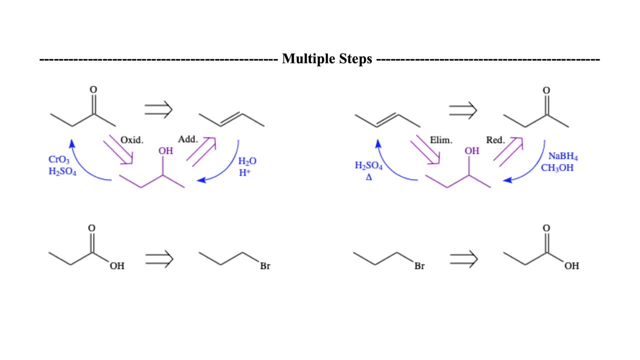 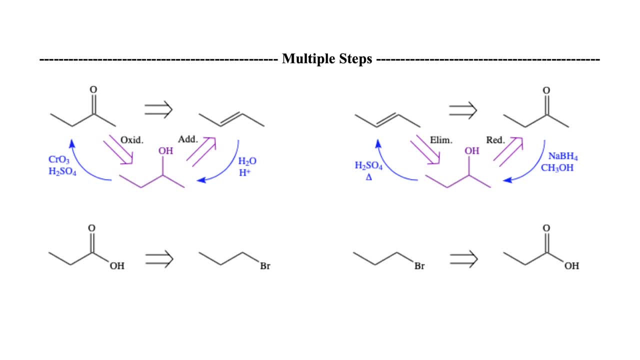 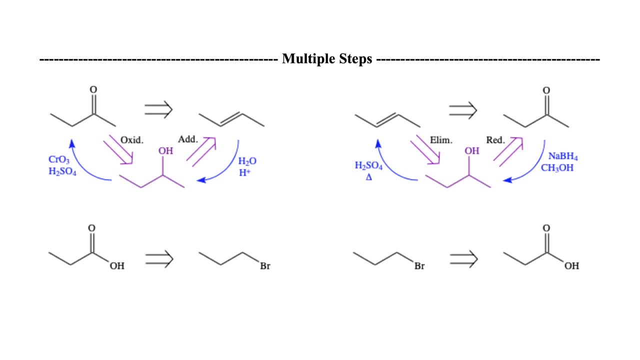 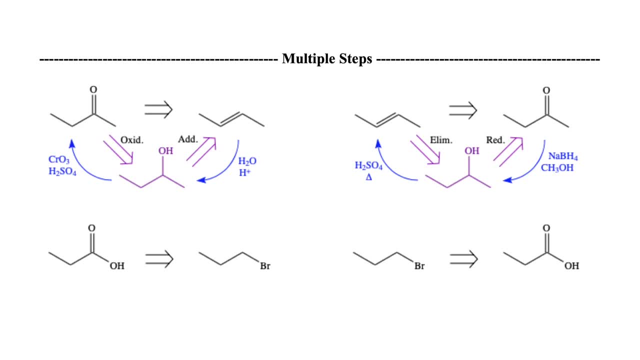 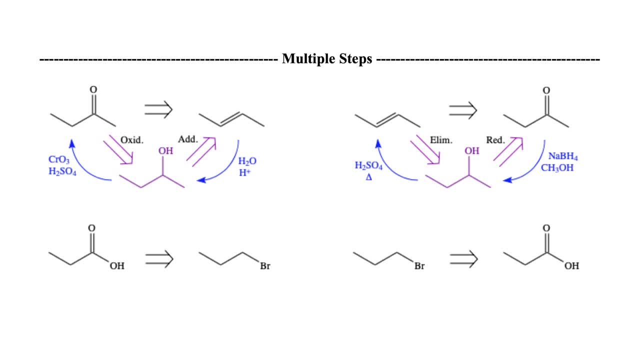 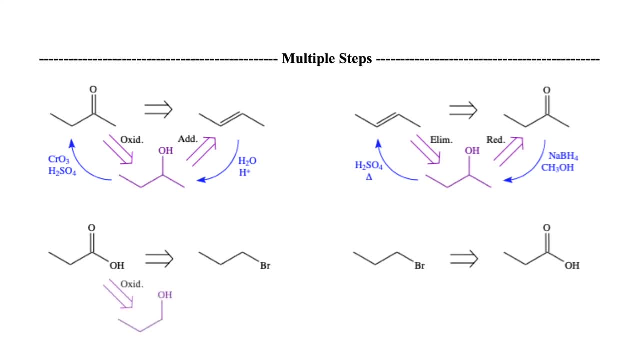 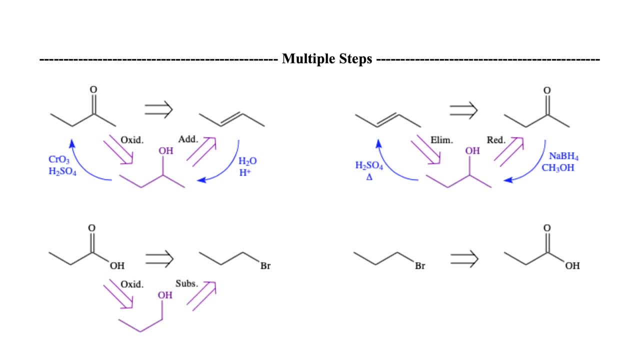 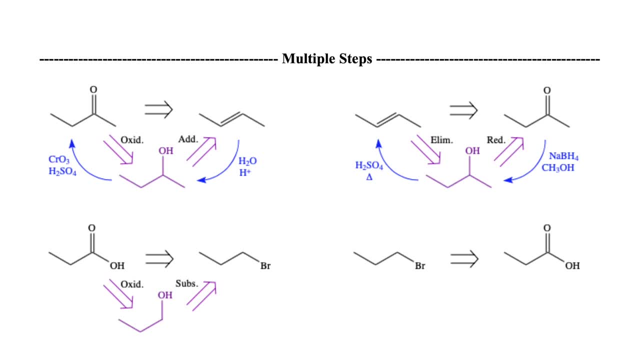 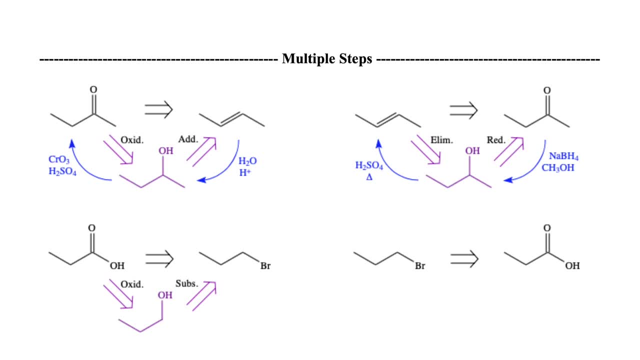 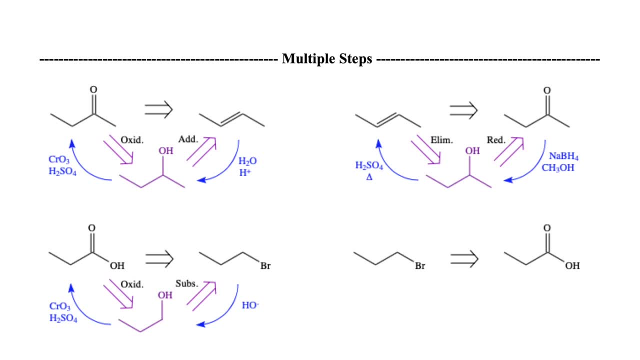 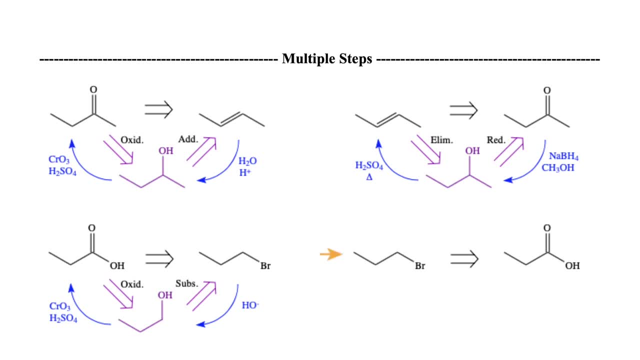 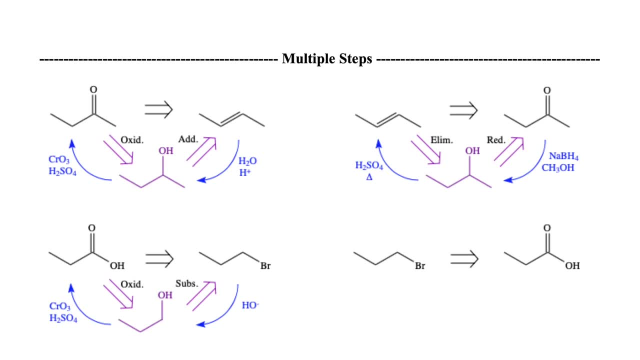 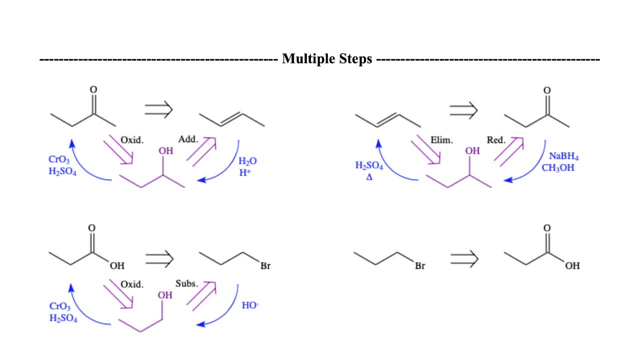 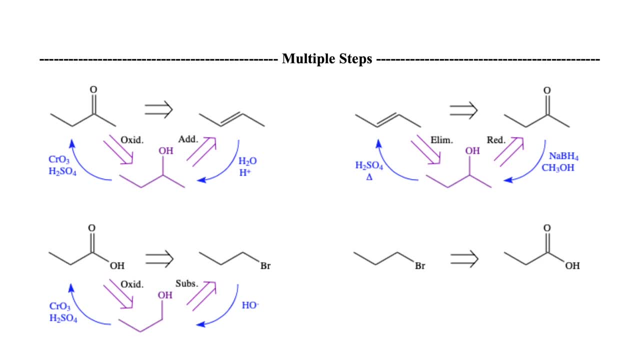 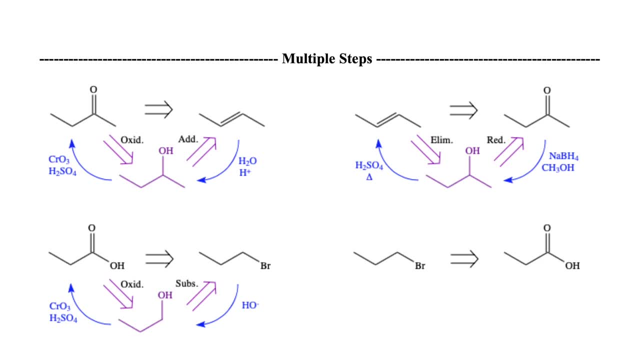 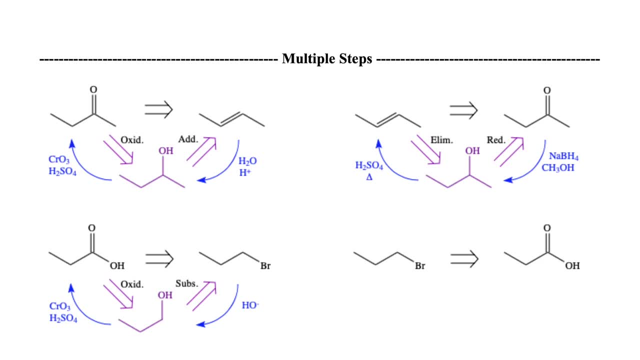 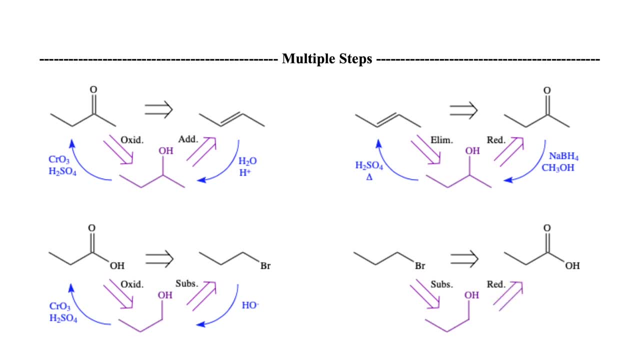 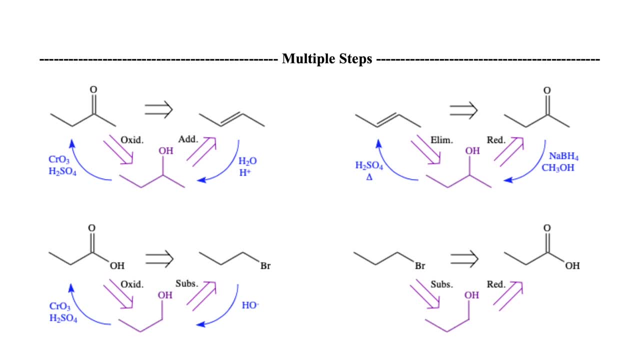 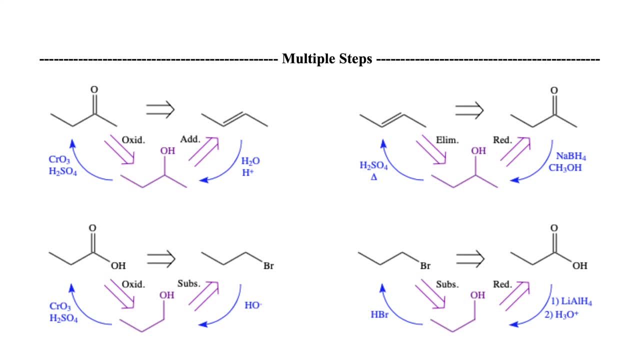 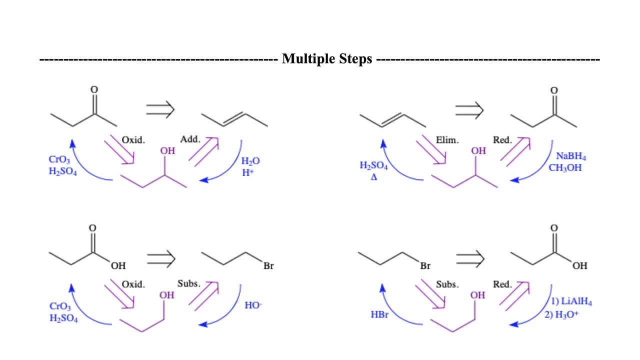 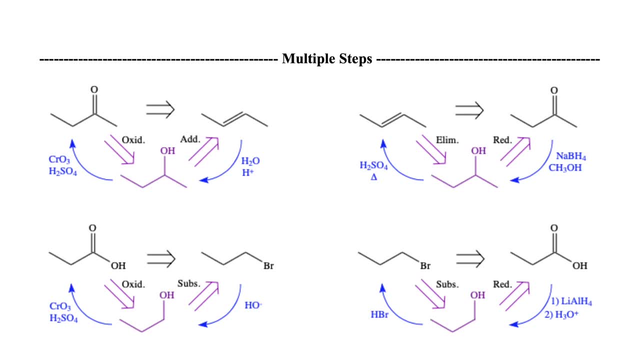 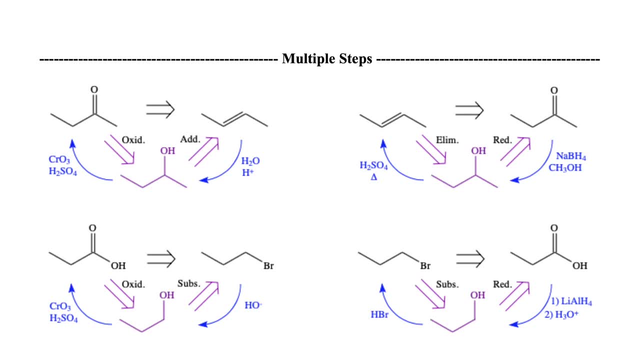 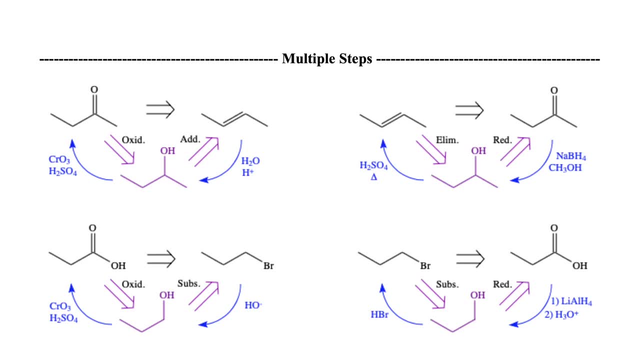 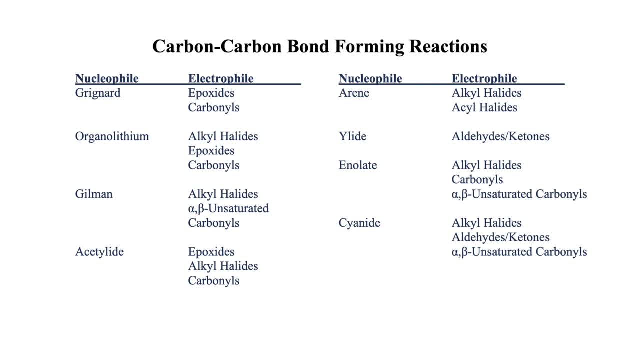 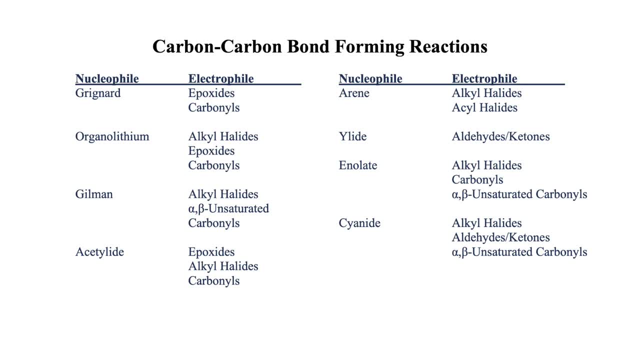 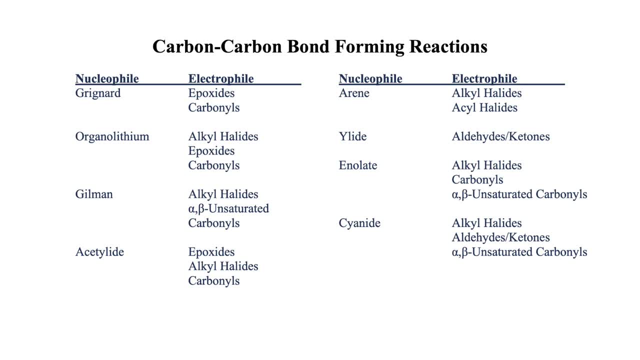 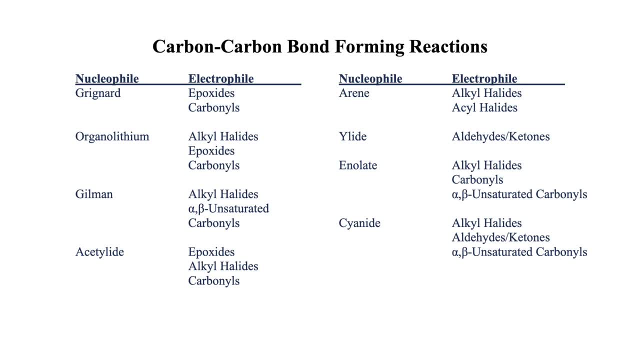 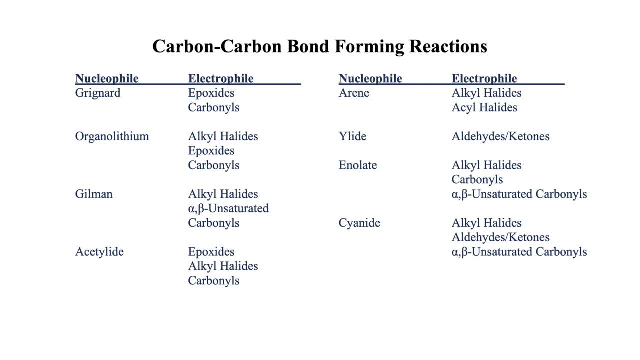 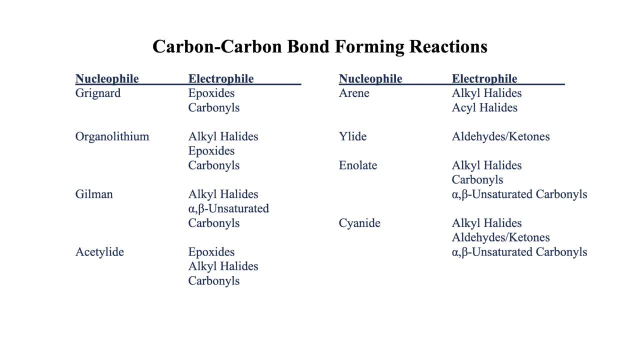 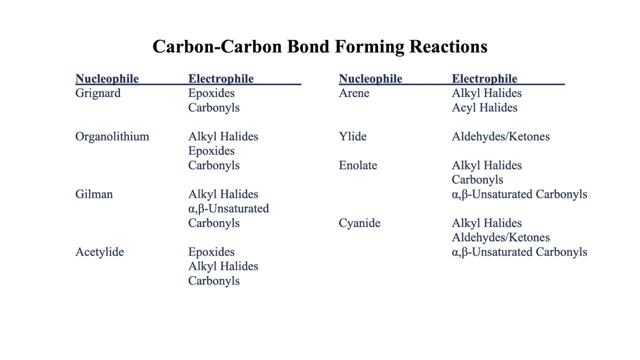 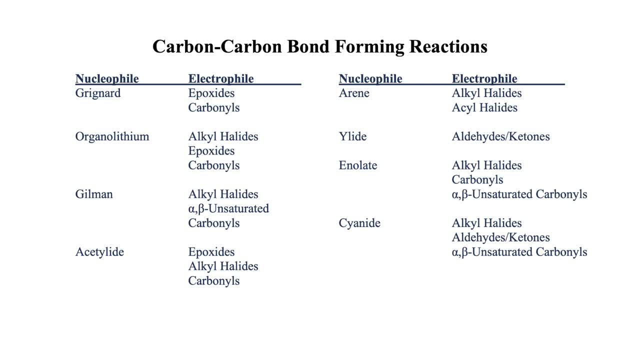 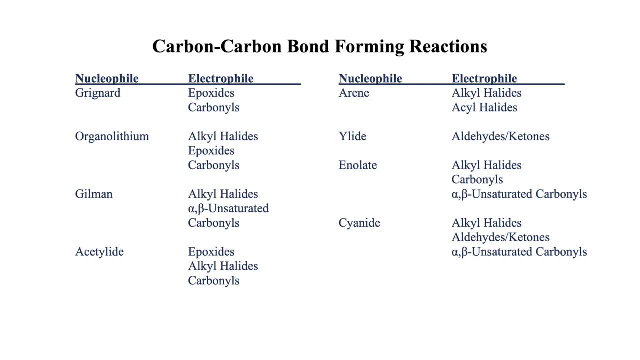 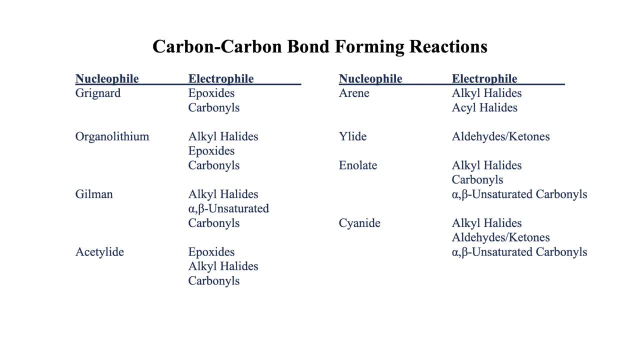 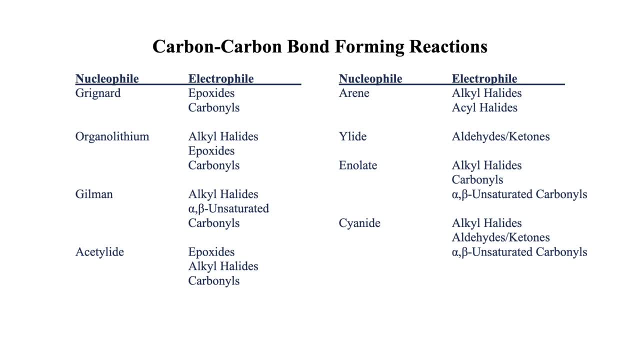 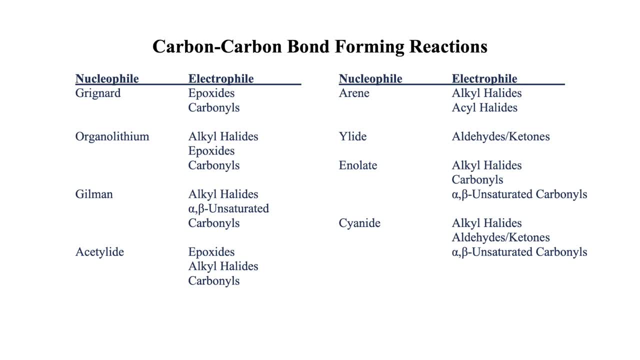 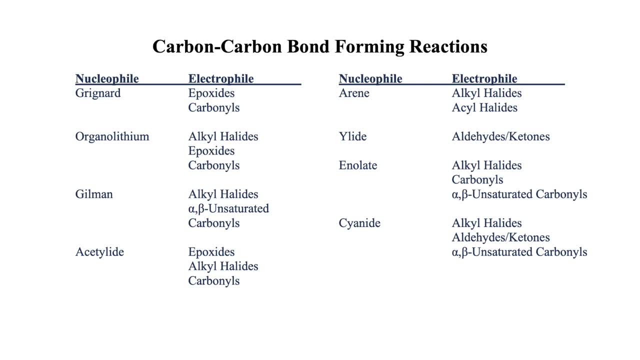 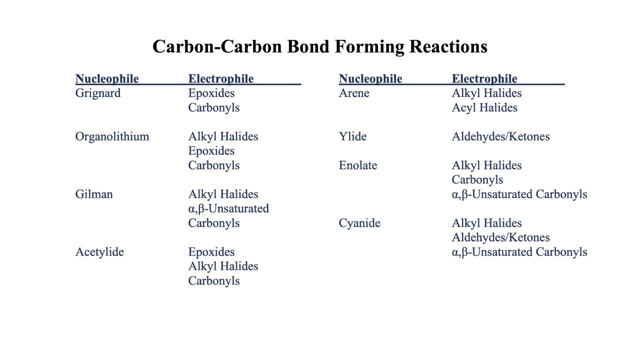 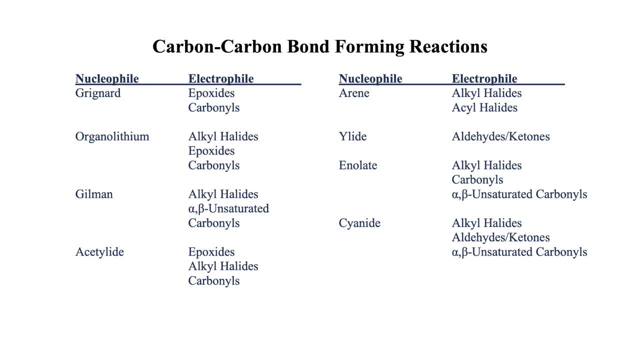 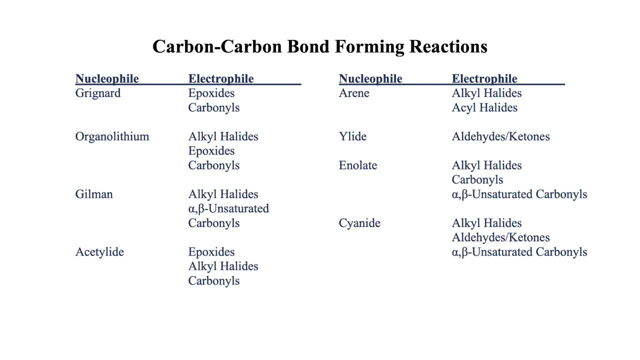 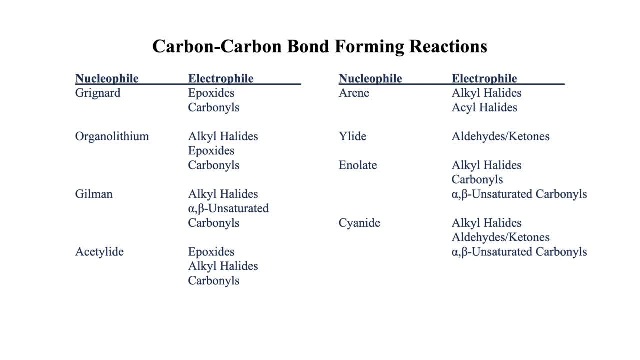 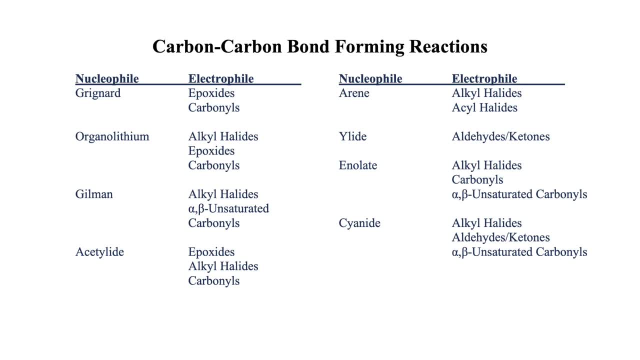 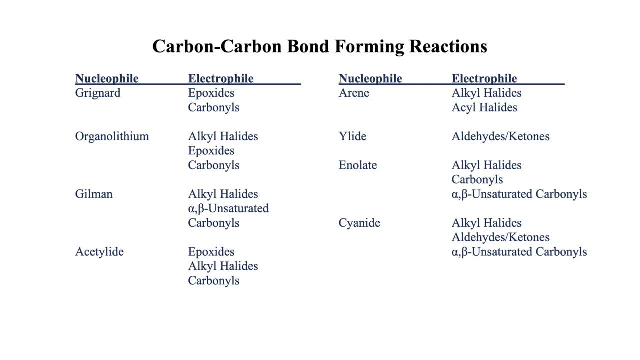 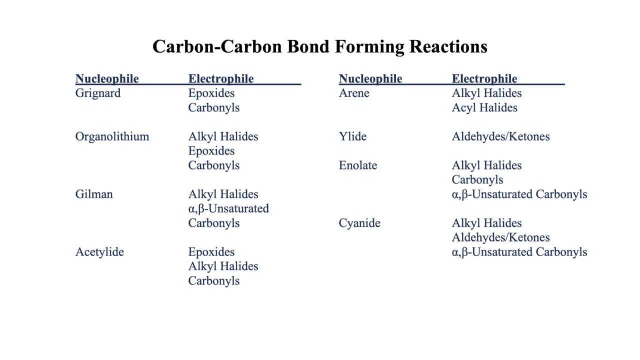 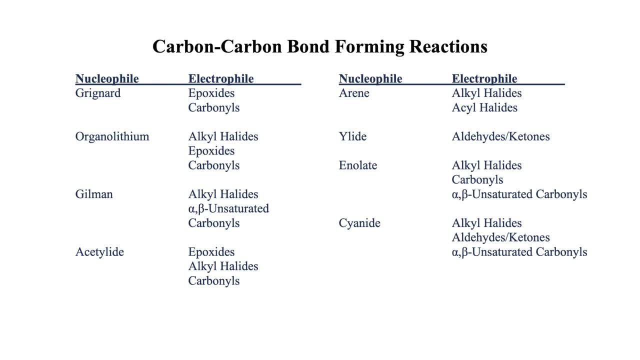 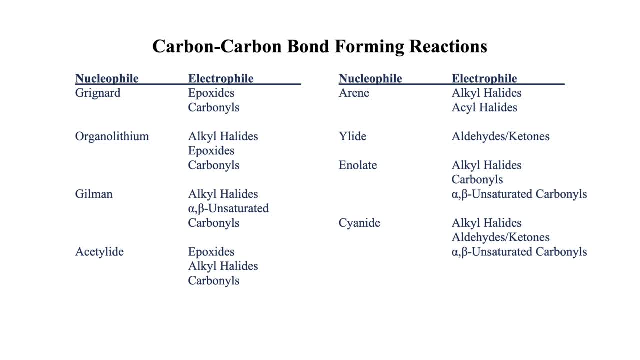 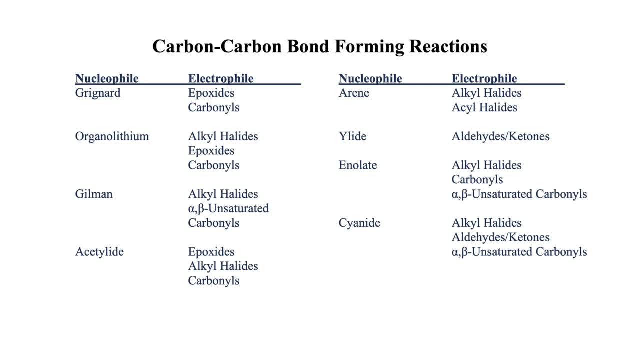 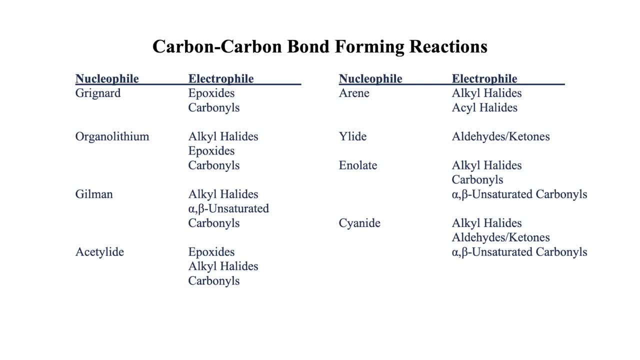 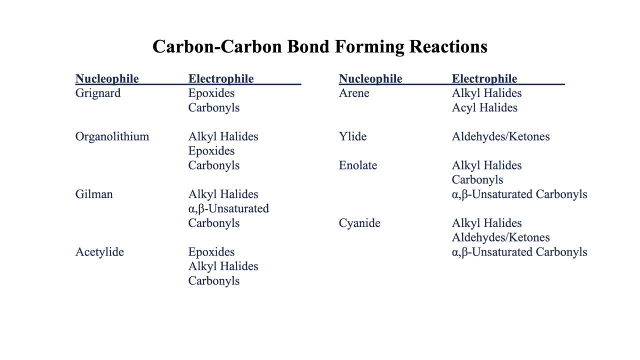 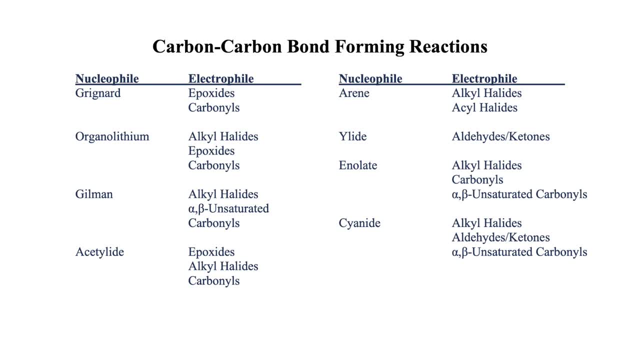 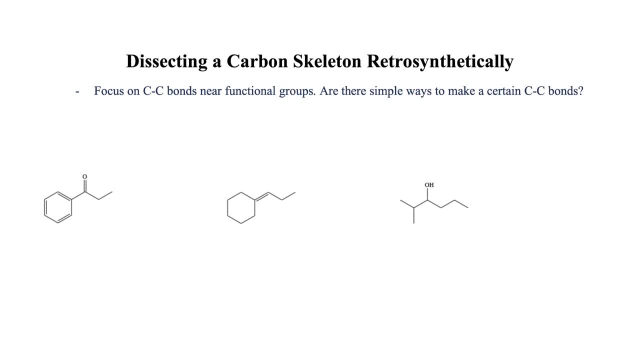 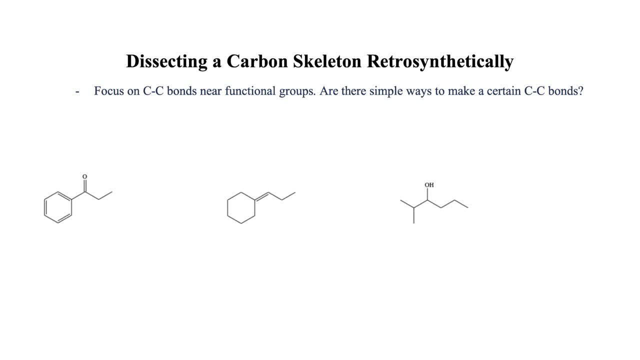 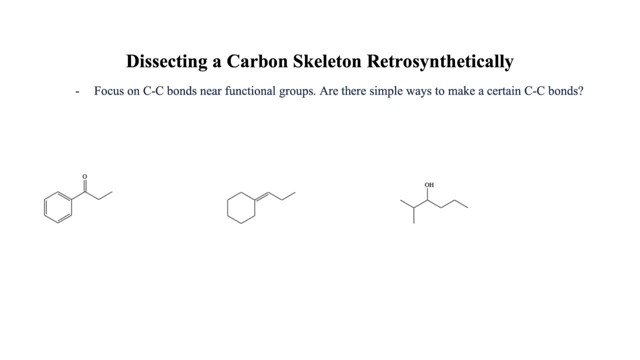 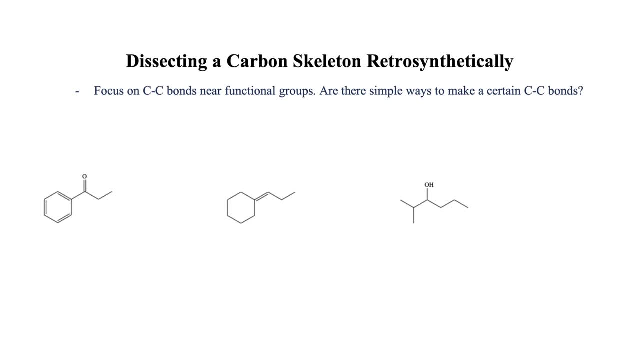 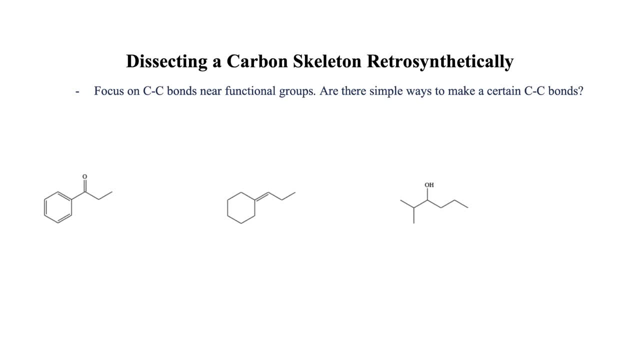 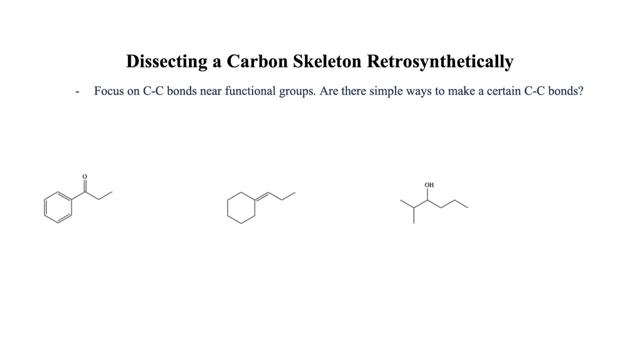 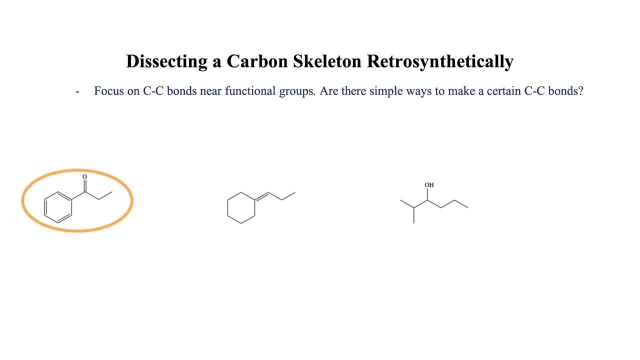 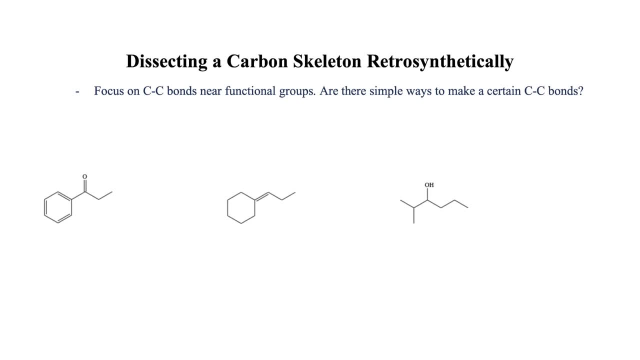 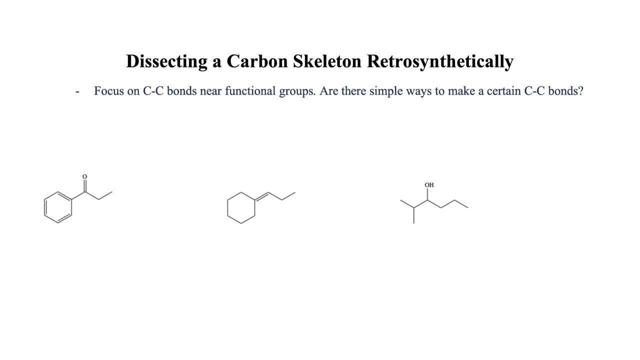 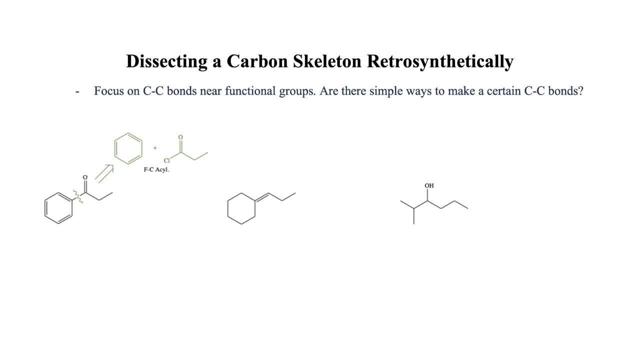 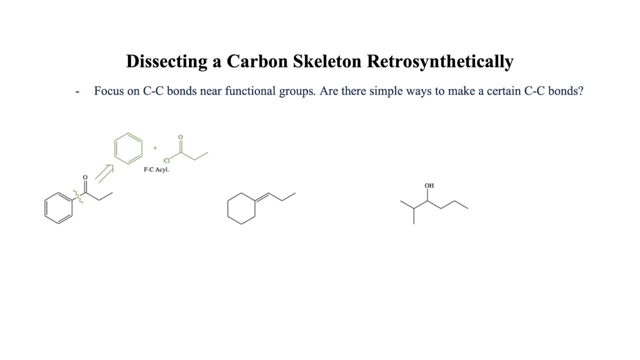 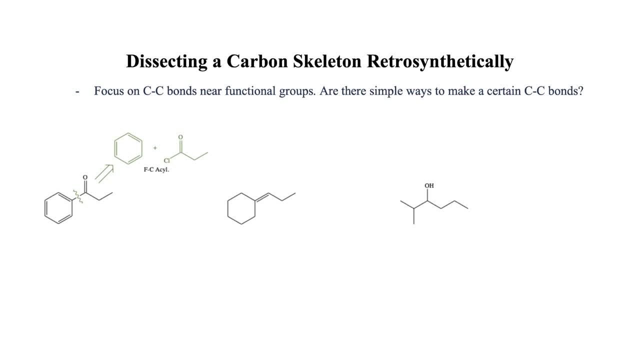 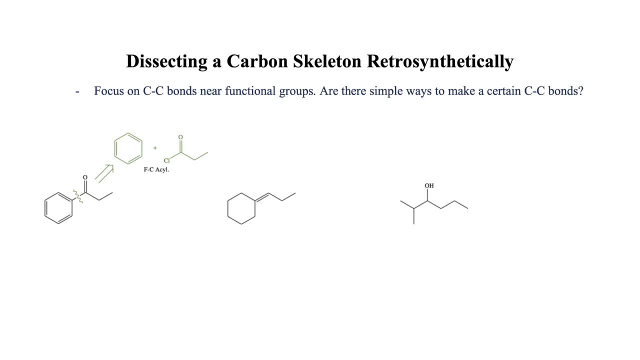 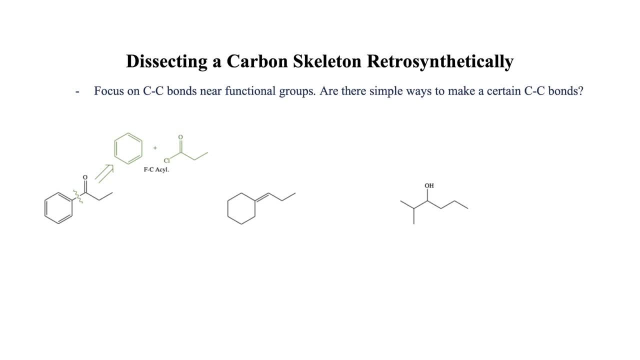 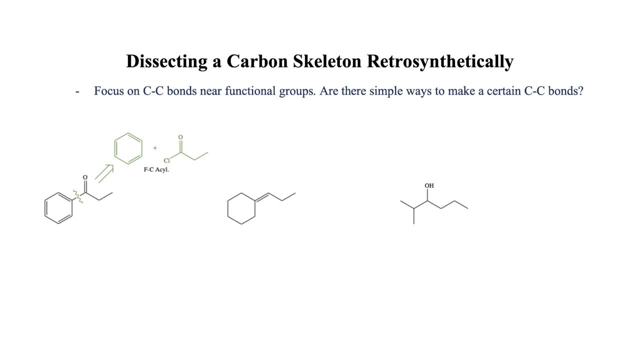 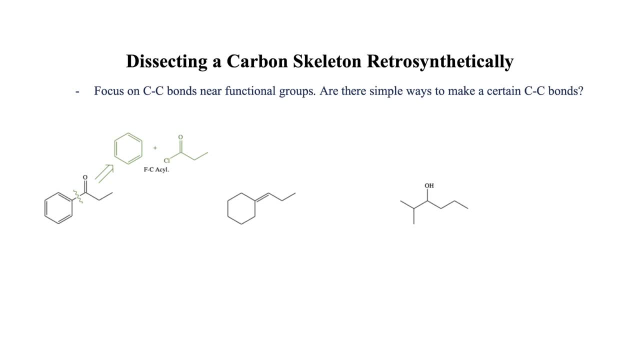 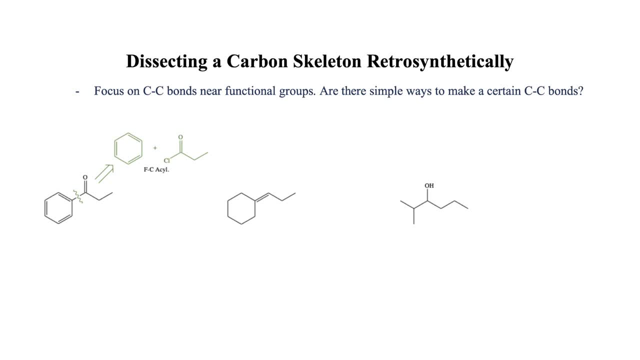 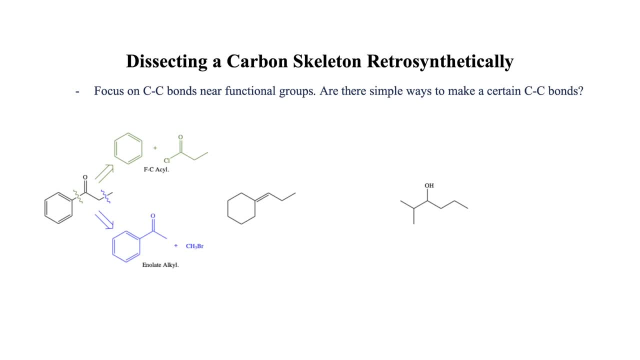 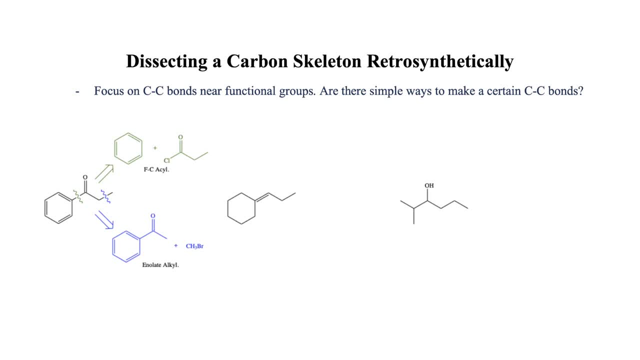 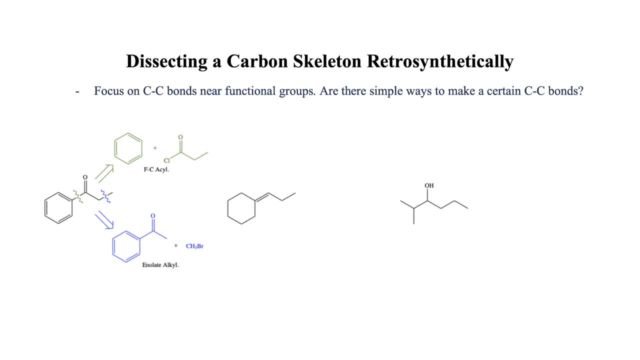 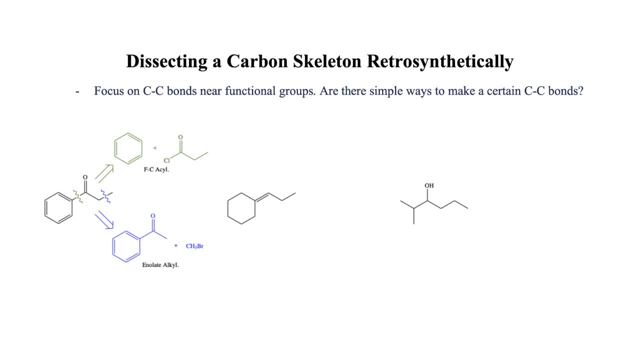 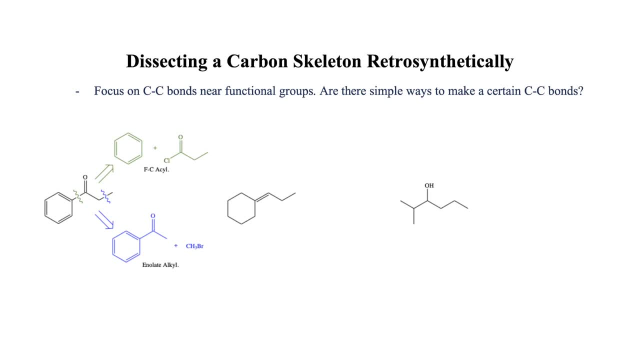 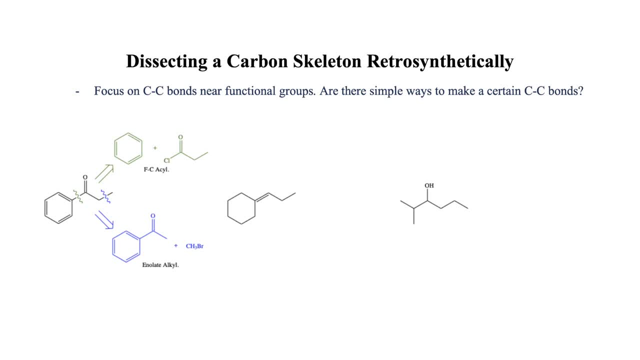 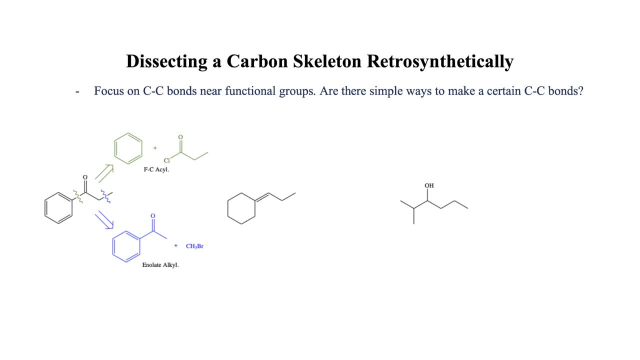 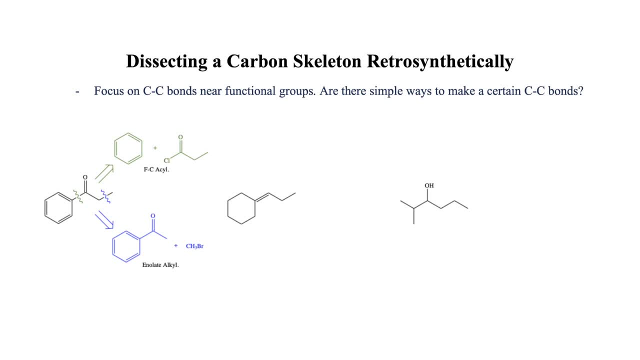 Hydration with water onto the alkene. Hydration with water onto the alkene to two larger chunks. that's a better retrosynthetic analysis. So let's take a look at this next one. It's a little more challenging. So here I have an alkene. 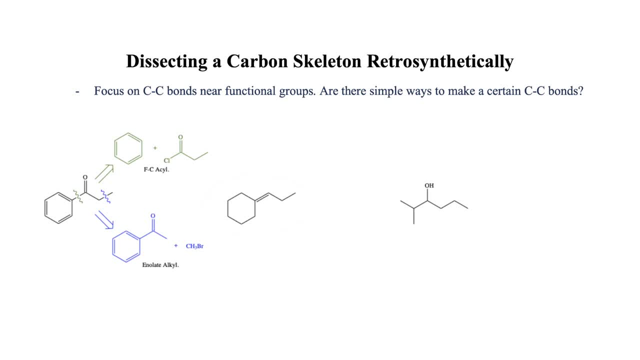 That's my functional group. So what kind of carbon-carbon bond-forming reactions result in having an alkene in the product? Well, I can think of a few. actually, We can have technically, things like Gilman couplings can have alkenes involved. 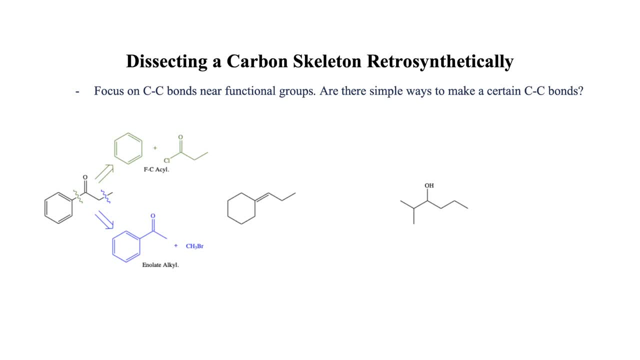 You can have aldol condensations, because the elimination in an aldol condensation results in the formation of an alkene. But we don't have a carbonyl here, right, Remember, aldol condensation requires that the product be an alpha-beta unsaturated carbonyl. 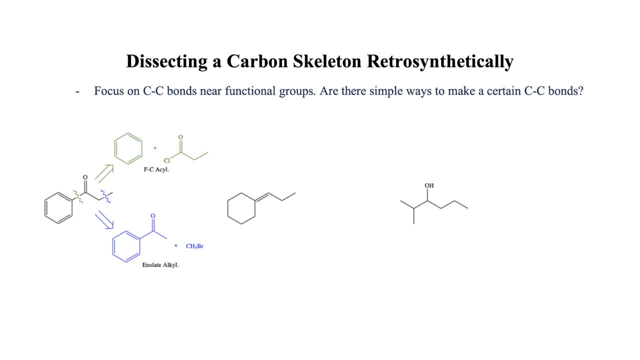 and we don't have a carbonyl here. We do know of one carbon-carbon bond-forming reaction that actually makes alkenes, and that is the Wittig reaction. So if I take this alkene and I split it in half, 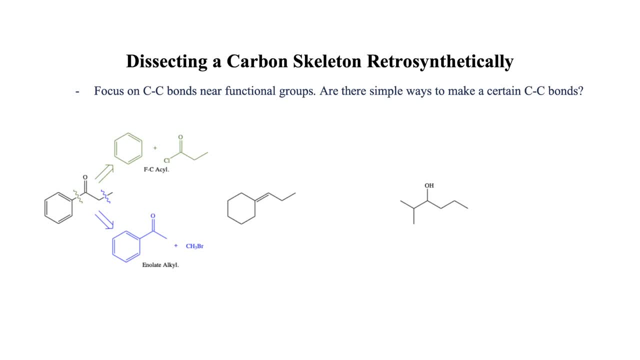 think about what a Wittig reaction is. It's the reaction of a carbonyl like an aldehyde or a ketone and a nucleophilic illid- One of the little quirky things about an alkene, when you're thinking. 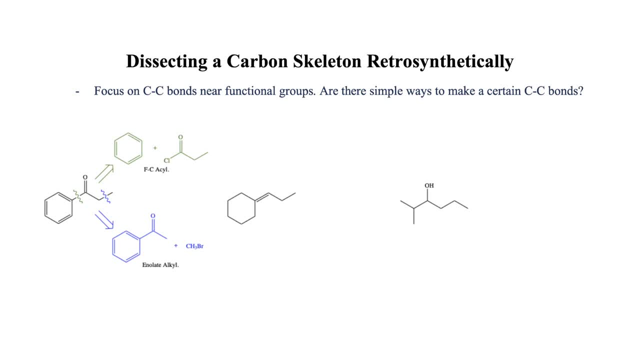 when you're thinking about making that bond through retrosynthetic analysis via a Wittig reaction, it could have come from two possible pairs of reagents. So let me show you what I mean If I break this carbon-carbon bond. one half of that had to be the illid. 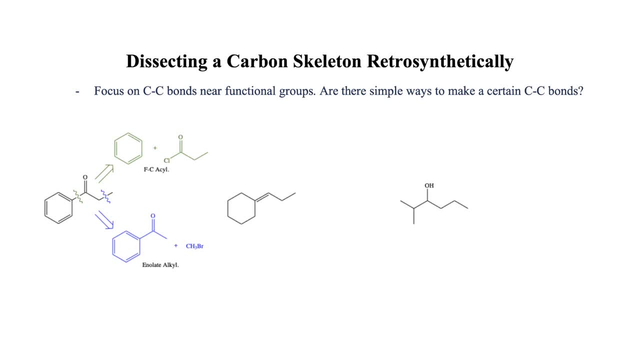 and one half of that had to be the carbonyl. So if I place the illid on the cyclohexane piece and the carbonyl on the propyl piece, then these are the two molecules that I get and they would react together. 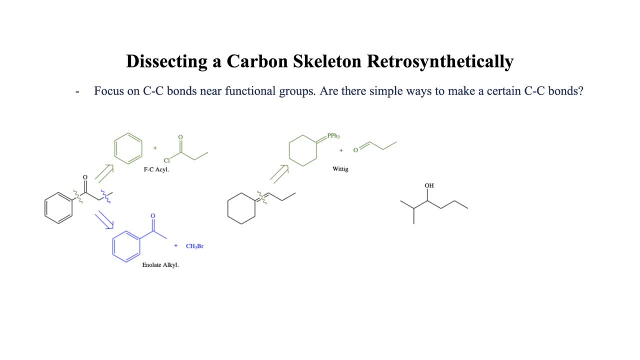 to make that particular alkyl. But I could have done it the other way around. I could have chosen, when thinking retrosynthetically, I could have chosen- to put the carbonyl on the actual six-membered ring and then the illid onto the three-carbon chain. 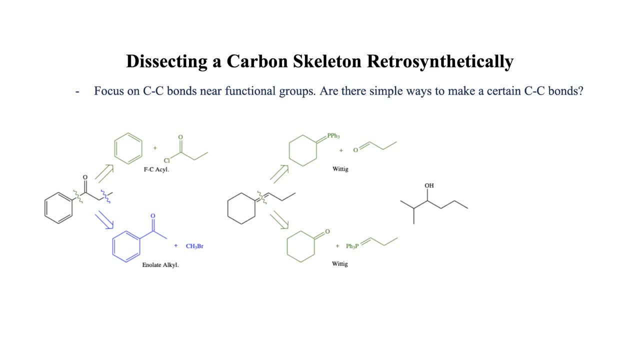 and that would give me these pieces here. Really, at this point both are perfectly valid analysis right. I mean, the aldehyde would probably be more reactive. This top reaction might be a little bit better, but either one is viable. 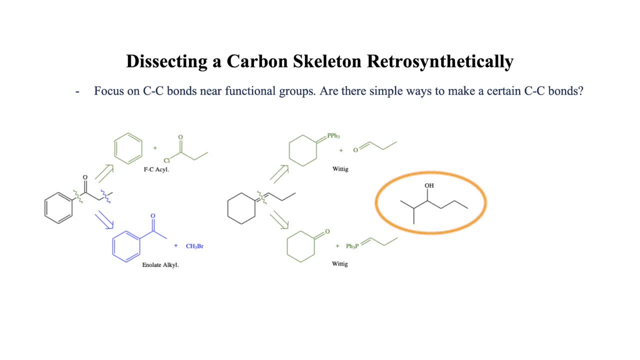 All right. so this next example is a little bit more involved, because there's actually a lot of people and there's actually a lot of possibilities here. So here I just have an alcohol. So what kinds of carbon-carbon bond-forming reactions? 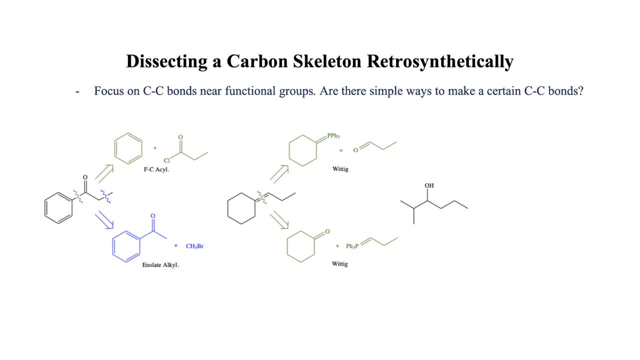 result in an alcohol in my product. Well, a lot actually. The first thing that comes to mind certainly is organometallic reagents, reacting with particularly aldehydes and ketones, But other things could be an aldol addition. 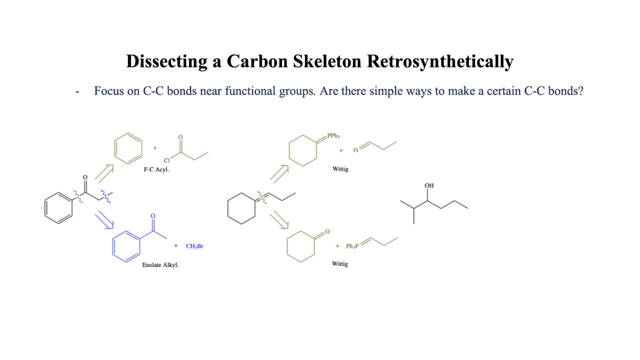 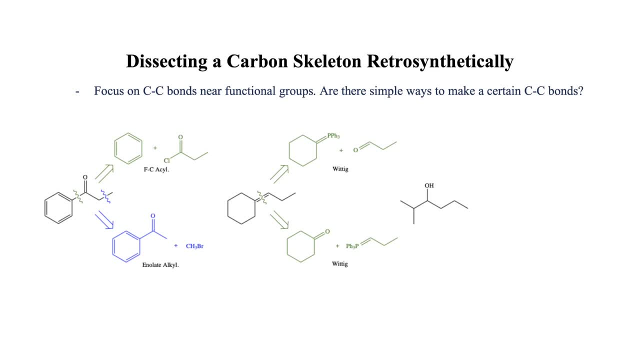 Right, I don't have a carbonyl in my product here, so I think that's a lot less likely. So let's take a look at this, If we were going to analyze this retrosynthetically. my functional group is this: alcohol. 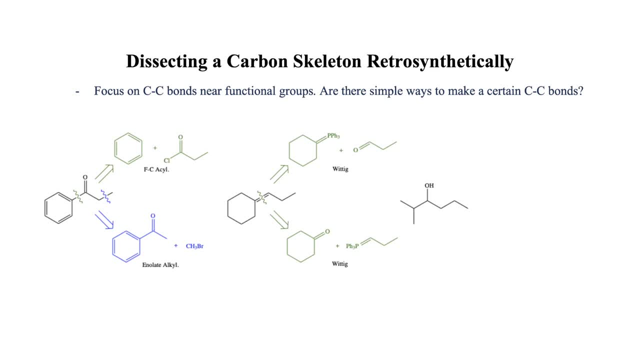 Now the carbon of that alcohol has electron deficiency, right, And I know that if I were going to react this to make an alcohol via, say, an organometallic reagent attacking it, that would have had to have been a carbonyl at one point. 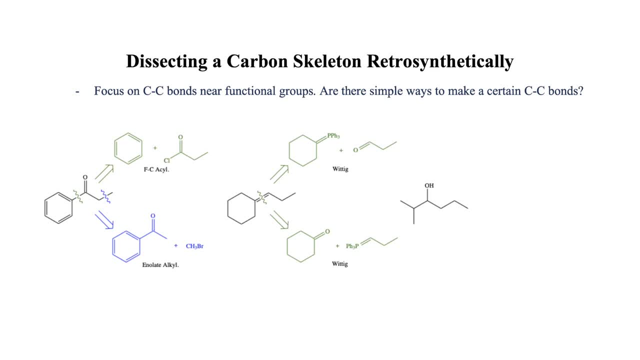 When the organometallic attacks the carbonyl, it breaks the pi bond and it results in an alcohol. So I actually could make either of the two bonds adjacent to the alcohol carbon If I cleave this bond, thinking retrosynthetically. 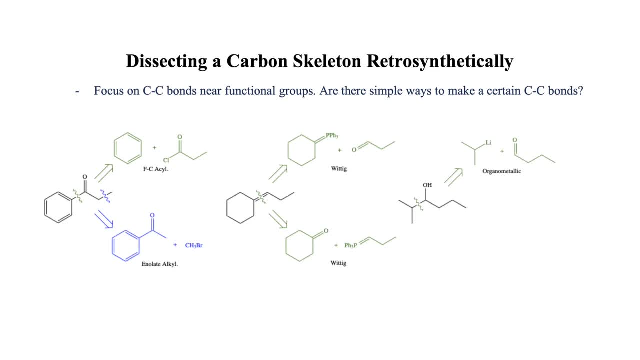 so if I make that bond, I would have had to have had an electrophilic carbon here, in other words an aldehyde, and then the other carbon on the other side of that bond would have had to have been an organometallic reagent. 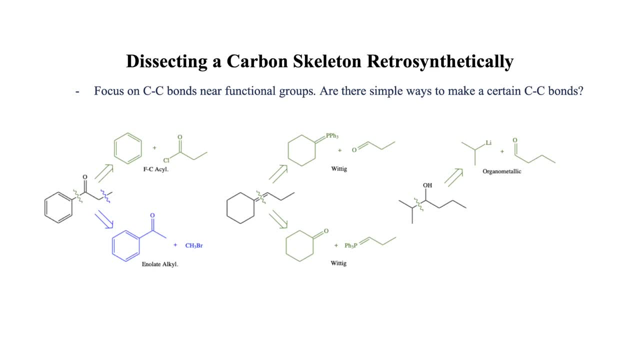 like a Grignard or an organolithium. These two molecules would come together and then, after protonation, go ahead and create that target molecule. I could again also make that other bond on the other side of the alcohol And really the chemistry is the same. 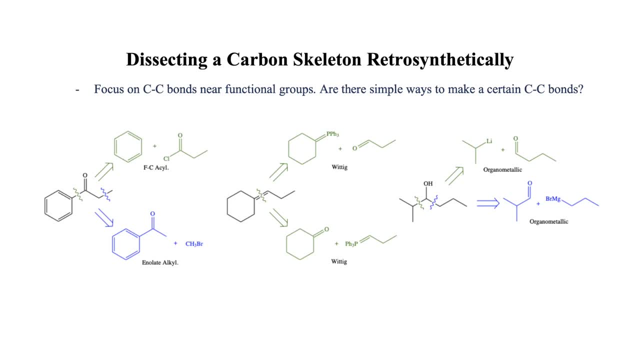 it's just the breakdown is a little bit differently. Again, the carbon with the O would have had to have been a carbonyl And being a carbonyl, it would have been attacked by a three-carbon chain organometallic. 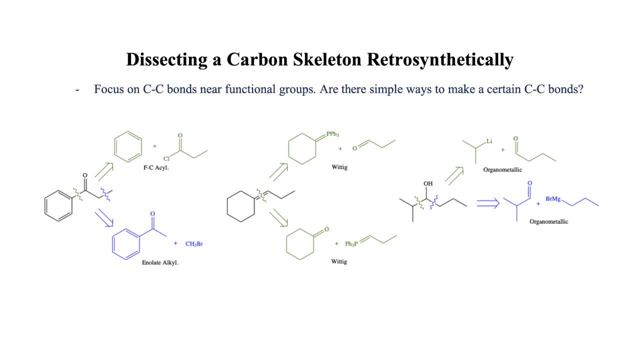 like a Grignard organ and organolithium, But those two molecules could have come together to form that particular bond. There's actually a third option here that's a little bit harder to spot because it's a little further removed from the actual functional group. 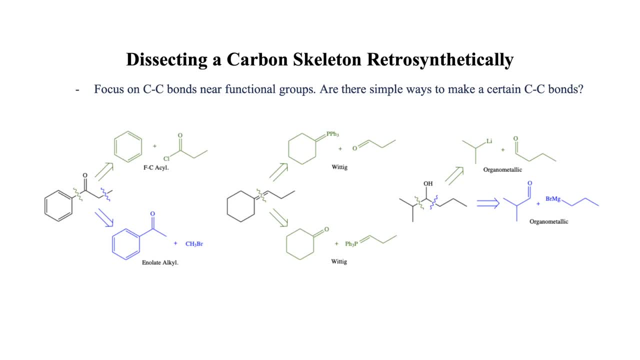 But we did learn that organometallics can react with epoxides in a ring-opening reaction. that also results in the formation of an alcohol, And that means that I could have actually also made this bond here broken in red. This is a little tougher to see. 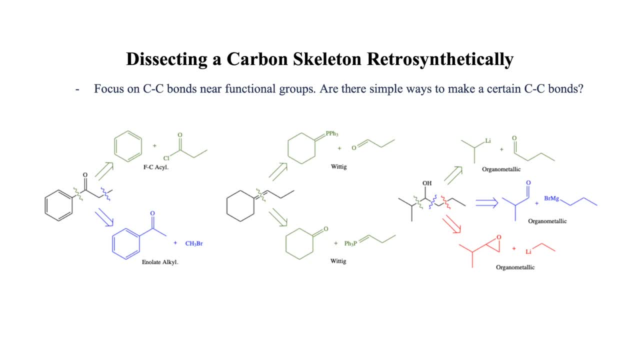 because now the electrophilic carbon is going to wind up being this carbon here, the left carbon of that carbon-carbon bond. Think about it: the alcohol in my product, that oxygen would have been attached to that carbon as well as to the carbon it's already bonded to. 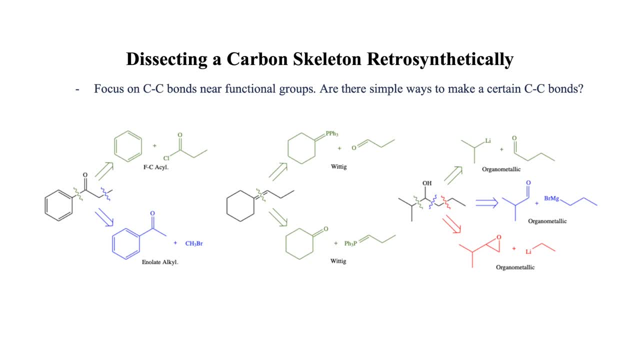 That would make a three-membered ring. that would make an epoxide. So it's possible to make this bond as well, reacting this epoxide with, say, organolithium, ethyl lithium. in this case, The ethyl lithium could attack. 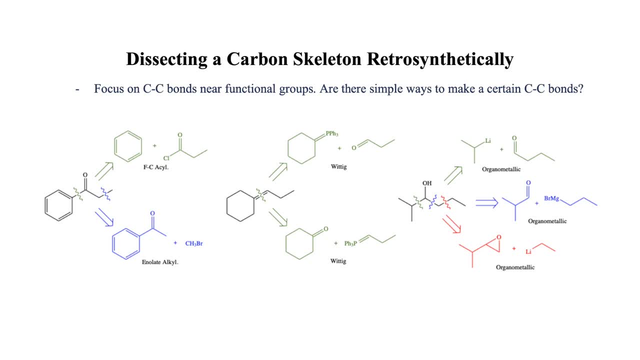 the less-substituted site of the epoxide, making that carbon-carbon bond and popping the ring open, ultimately getting protonated. So when you only have one functionality to focus on when you're looking at how to make the carbon-carbon bonds, 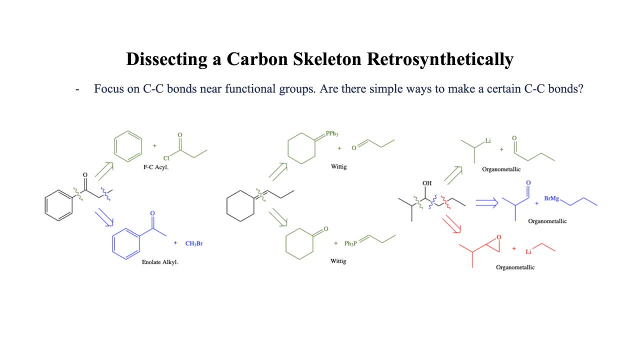 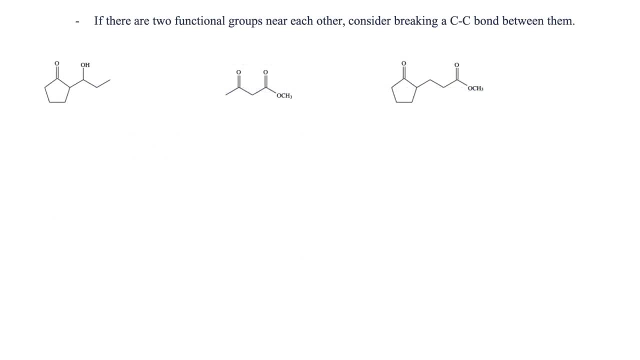 how to dissect that retrosynthetically focus in and around the actual functional group. Now, in some ways this actually becomes easier when you have multiple functional groups, or at least it can. Let's look at this, for example: I have two functional groups. 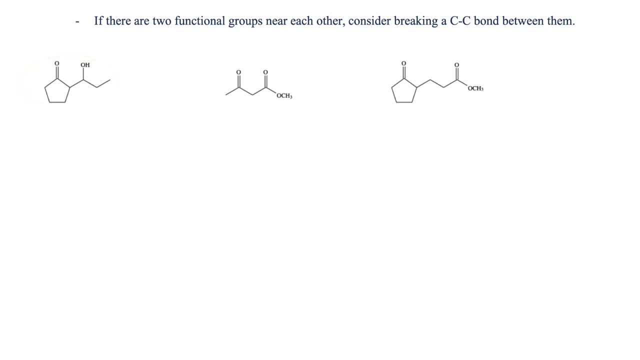 I specifically have a ketone and an alcohol. Now, a lot of times when you have two functional groups, you end up making the carbon-carbon bond or one of the carbon-carbon bonds between those two functional groups. In this case, I have a very kind of obvious way to go. 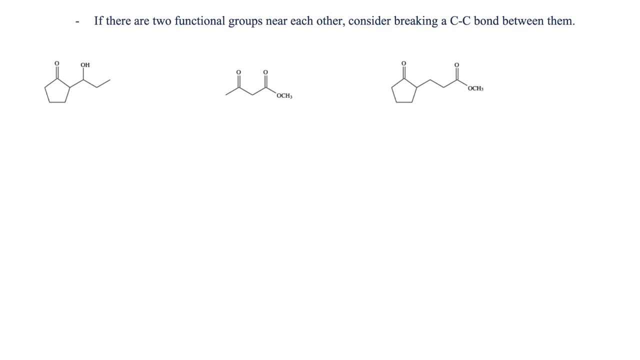 because I have a very specific functional pairing. What I have here is a beta-hydroxyketone, And any time I see a beta-hydroxyketone I immediately think that could be made through an aldol addition, An aldol reaction, and remember. 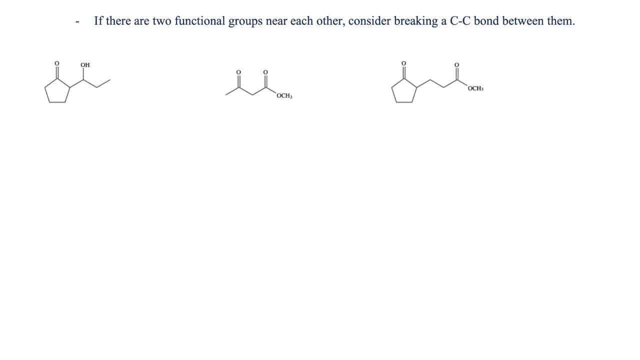 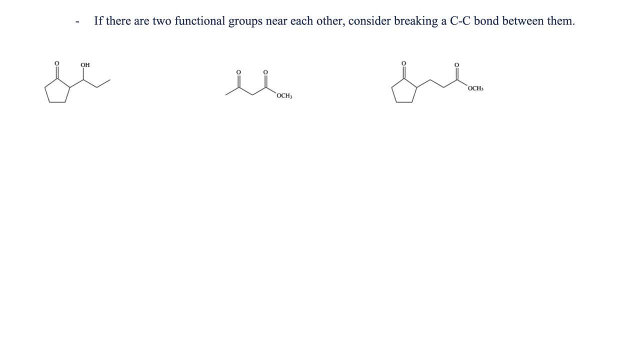 So you wind up making a bond between the aldol and the ketone, And then whatever the carbonyl was that you attacked. So, thinking retrosynthetically here, it would be this bond I would cleave, resulting in reacting cyclopentadone. 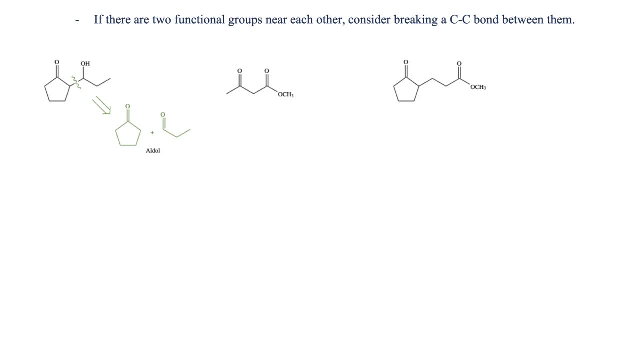 and propanal. in this case I would enolize the cyclopentadone with, say, LDA and then react that with propanal. So here's another one. I've got two functional groups, So I'm already thinking it's probable. 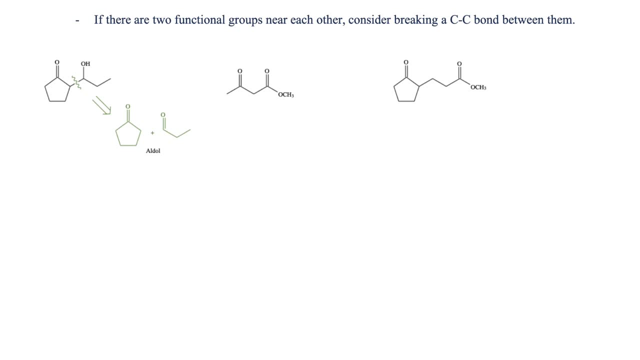 that I'm going to wind up making one of the two bonds in between those functional groups What I'm trying to think of. how would I make this structure? What bond would I break? thinking backwards, Well, I see that again, this is a very special functional pairing. 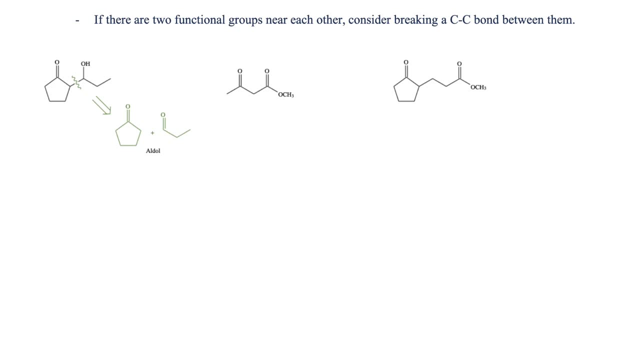 This is a beta-ketoester, And beta-ketoesters can be made through Clisen condensations, And in a Clisen condensation you wind up making a bond between the alpha carbon of an ester and the carbonyl of another ester. 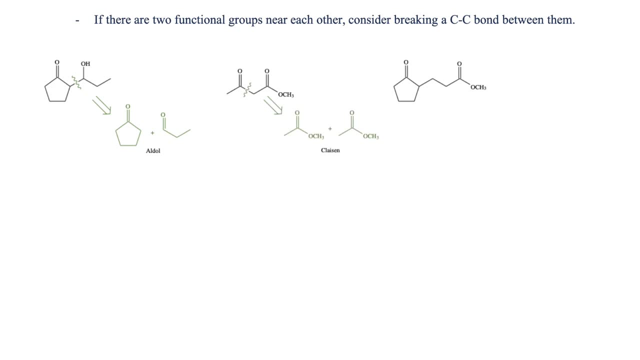 And that means that, thinking backwards, it would be this carbon-carbon bond that would actually be made. So, breaking that bond, I would wind up with one side of it being an ester and then the other side would have been an ester, right. 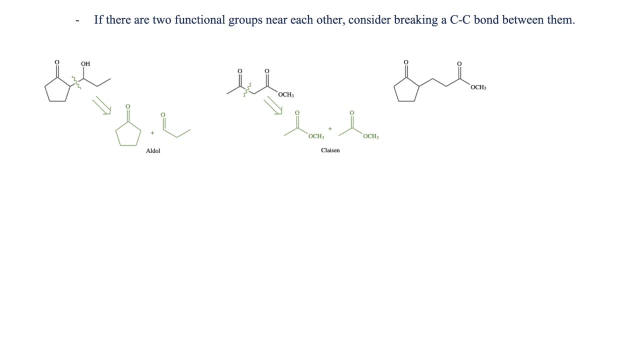 That carbonyl would have had a leaving group attached to it that would have been displaced by the enolate from the other molecule. So in this case it's actually just two molecules of methyl acetate reacting together. One would get enolized. 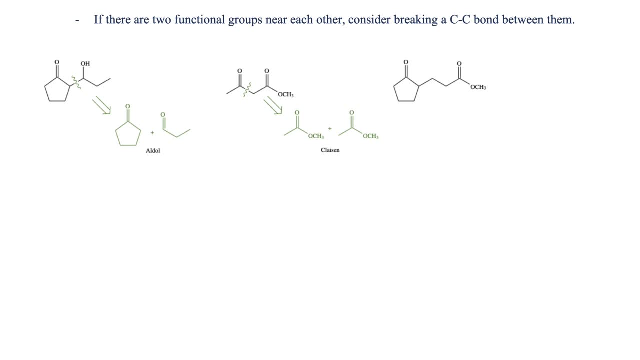 and that would attack the other one, doing a substitution reaction. So here's a third example when I have multiple functional groups. Here again I have a ketone and an ester, but it's not the same relationship, right? They're further away. 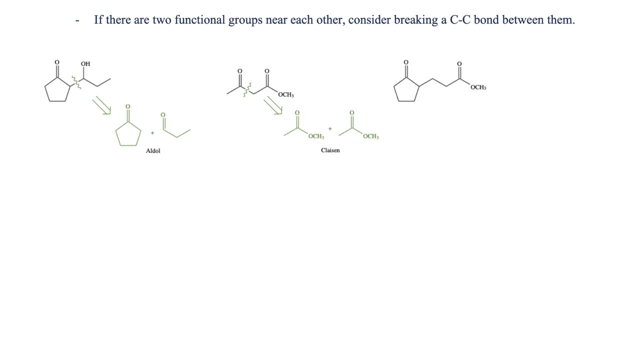 So again, I'm already thinking: let's go ahead and try to see if we can make one of the bonds between those two functional groups, And in this case I have yet another kind of special functional group pairing, because what I have here is a 1,5-dicarbonyl. 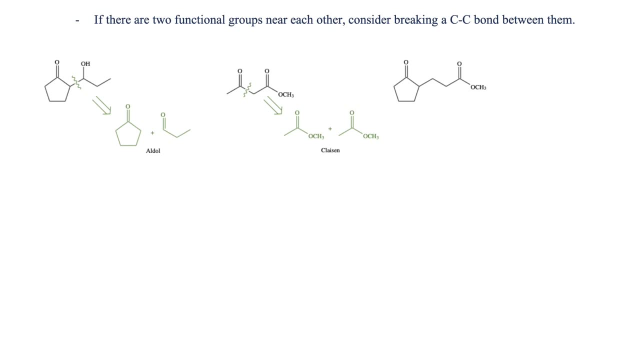 And 1,5-dicarbonyl, as you might remember, can be made through Michael additions. This can be a little bit tougher to kind of visualize. I think There's a lot of bonds in between those two carbons. 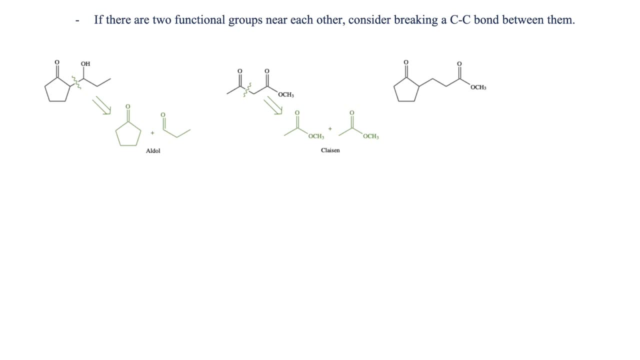 those two functionalized carbons, So it can be a little harder to see. But in this case, what I'm going to do- remember what a Michael addition is- You form an enolate of one carbonyl and then attack an alpha-beta unsaturated carbonyl. 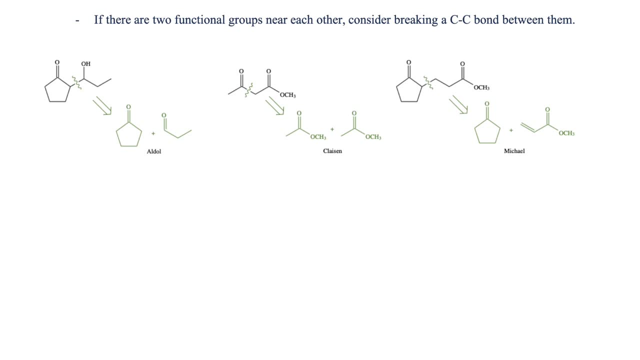 So that means that I could have made this carbon-carbon bond. I would have had cyclopentanone as my enolate source, And then this other piece would have had an alkene in place, giving it alpha-beta unsaturation. 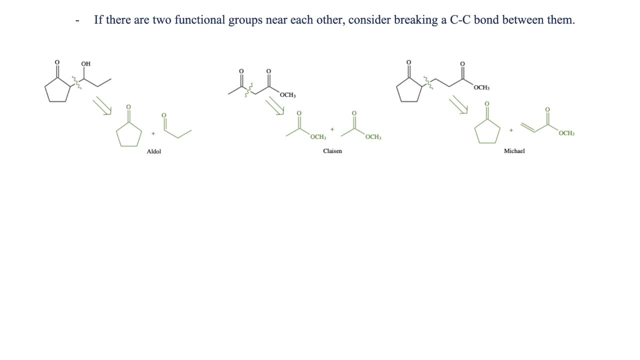 In other words, I could have made this from cyclopentanone. reacting with this particular alpha-beta unsaturated ester, I would enolize the ketone. It would then do a conjugate attack on the alpha-beta unsaturated ester, doing a Michael addition. 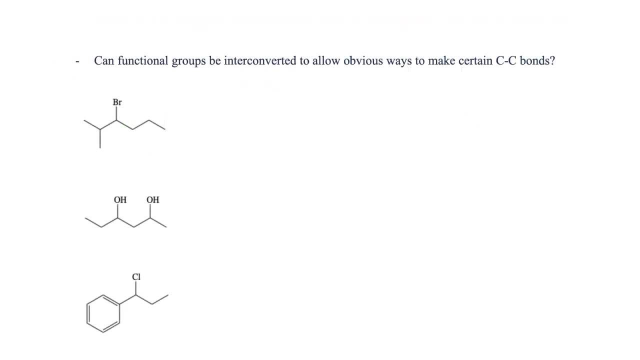 So let's make things a little more interesting, Let's bump up the difficulty level a little bit, Because sometimes you're going to see a target molecule that has a functional group that really doesn't call attention to itself in terms of hey, I can make a carbon-carbon bond. 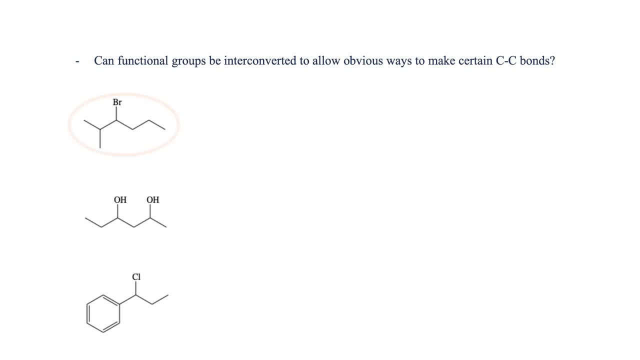 that results in this kind of functionality. So here's an example: I've got this alkyl halide And there aren't really any carbon-carbon bond forming reactions that I know of that can actually result in an alkyl halide specifically. 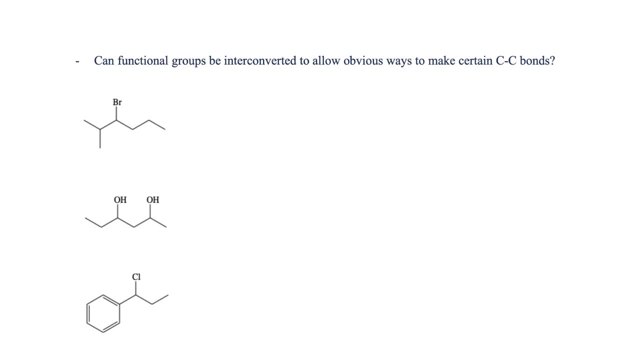 So this is where we can kind of pull together everything we've talked about here. What we're going to need to do is think in terms of functional group interconversion that then sets up one of our carbon-carbon bond forming reactions. When I see this alkyl halide, I immediately think: oh, that alkyl. 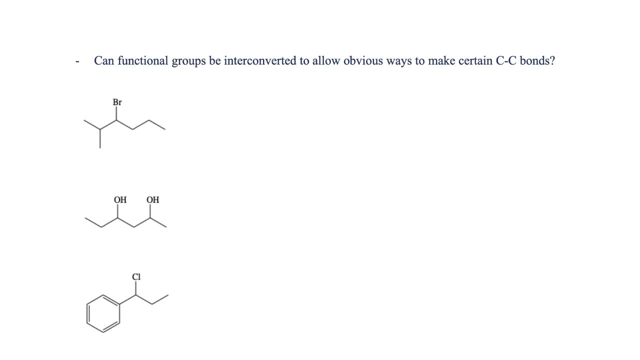 halide is junk. It's just as good as an alcohol, Because I can make that alkyl halide from an alcohol in one simple little step through a substitution, And I know a bunch of carbon-carbon bond forming reactions that can result in an alcohol as my product. 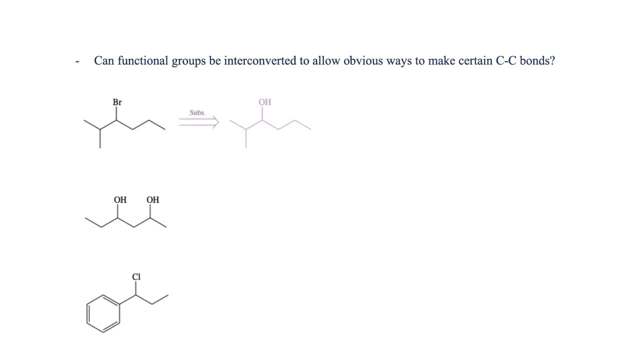 So, thinking retrosynthetically here, I get rid of this halogen, I do a substitution. This halogen, this alkyl halide, could have come from this alcohol And you might recognize this alcohol. It's one of the examples that we talked about a little bit. 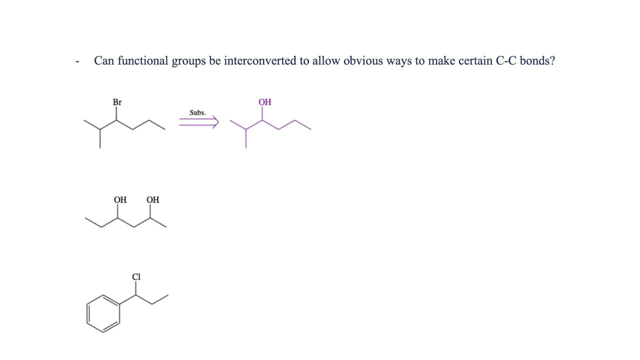 earlier, when we looked at breaking down uh carbon skeleton retrosynthetically, And that means that I could have made this particular alcohol via any of those three potential retrosynthetic analysis that we looked at earlier. So let's take a look at another example. 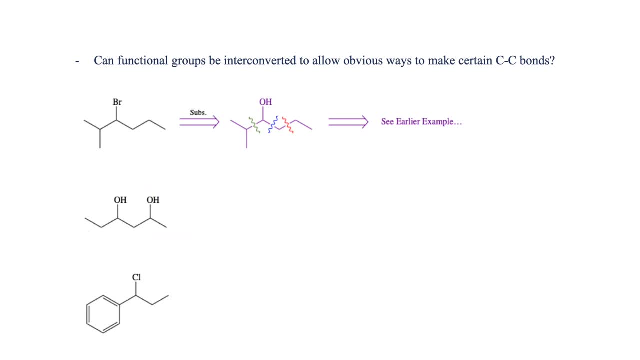 Here I've got a diol, a 1,3-diol specifically. Now I can make alcohols from carbon-carbon bond forming reactions And that's not a problem. But having two of them kind of is a problem. 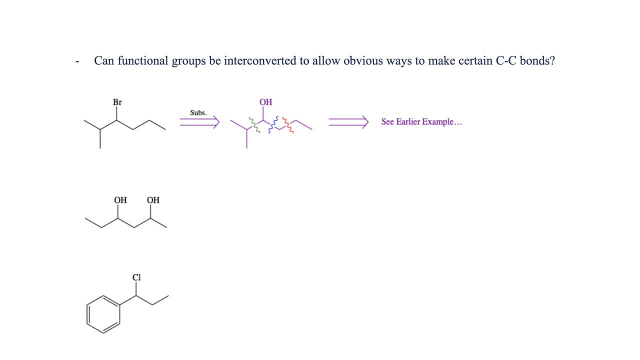 If you try to make one of these carbon-carbon bonds, that means you probably would have started with, say, an epoxide or a carbonyl on one of those alcohols, But the other alcohol would still be around And that's a problem if you try to do things. 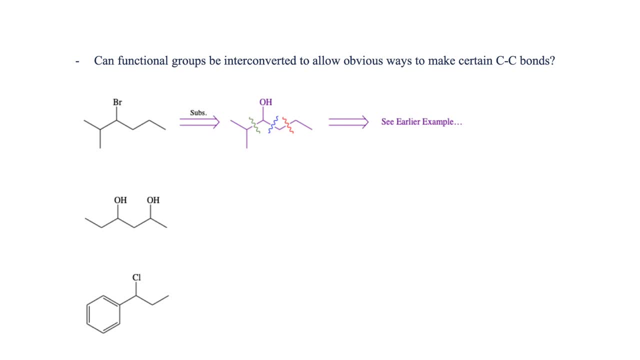 like organometallic chemistry, Because organometallics react with alcohols by destroying them, right? They actually react with the alcohol to get protonated. The organometallic will get protonated and it will be wrecked. 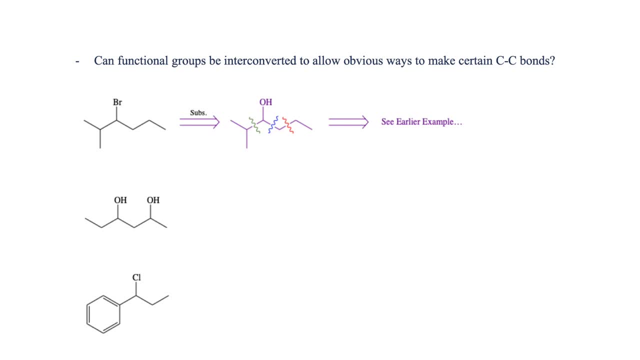 What I see here, though, is a functional pairing. that is almost something interesting. What I see is a relationship, a 1,3 relationship, between functional groups, specifically oxygen functional groups. When I see that, that 1,3 pairing- 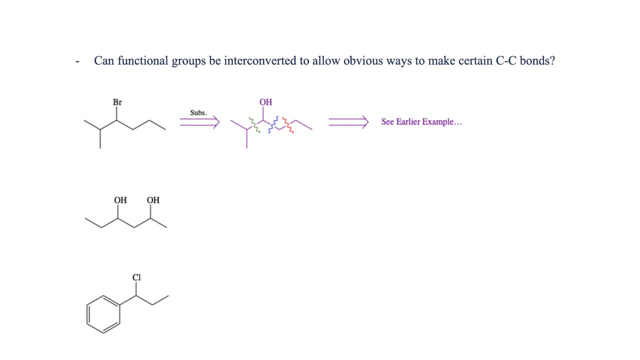 I think, oh, this could have come from an aldol, Because an aldol results in a 1,3 pairing of functional groups, specifically 1,3 pairing of oxygen functional groups. right A: beta-hydroxycarbonyl. 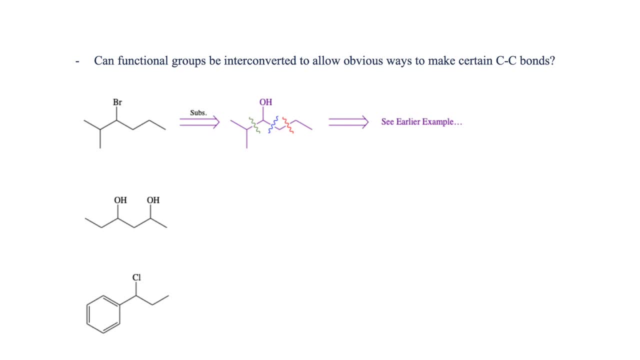 So, thinking retrosynthetically, I would look at this and say: well, what if one of those alcohols were at one point in time a carbonyl? Let's say this left alcohol. If I raise that up to a carbonyl, then what I have? 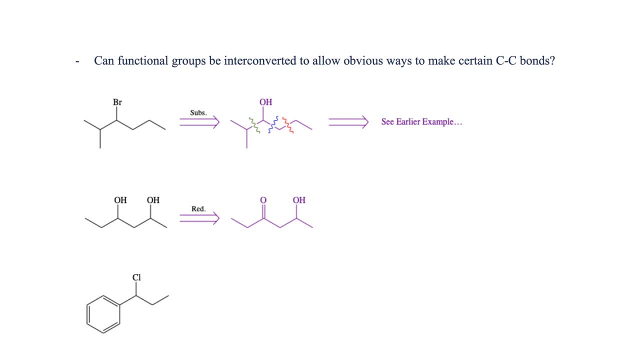 is a beta-hydroxyketone And that I could simply make via an aldol addition. That means I could make this particular carbon-carbon bond by reacting the enolate of this ketone with, in this case, acetaldehyde. 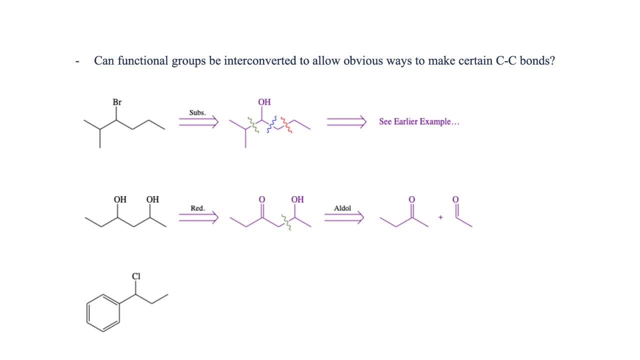 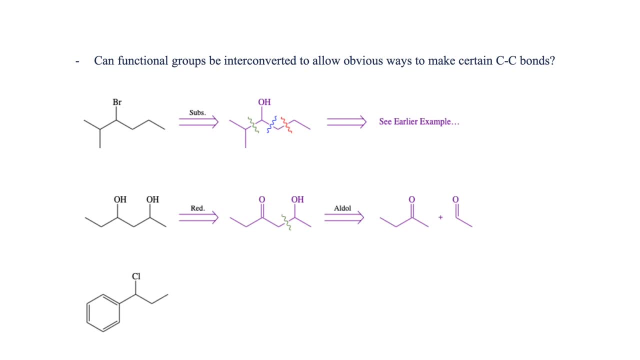 And that's what we're looking for And that set up a very, very obvious carbon-carbon bond forming reaction, because I see that beta-hydroxyketone that could be made from an aldol. I could certainly have gone through and done it. 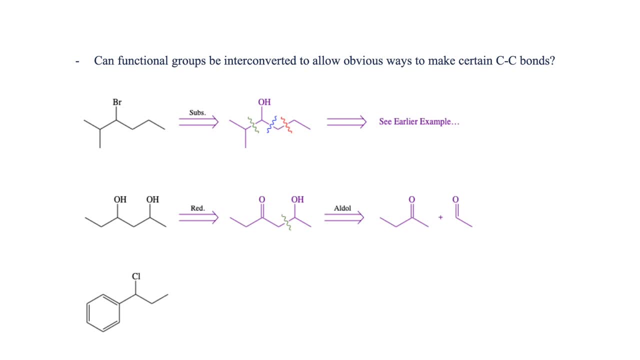 onto the other alcohol. I could have lifted the alcohol on the right to a carbonyl and broken it down again, thinking retrosynthetically- using an aldol addition, But I would have had a different carbonyl set as far as what I would start with, 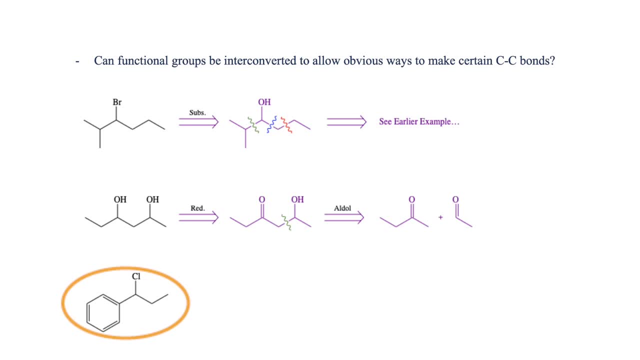 All right. so our last example. here I have an alkyl halide And again alkyl halide. You can think about alkyl ex cooks using alkyl halides as synthetic targets are a little bit tricky when you're starting to think in terms of making carbon-carbon bonds. 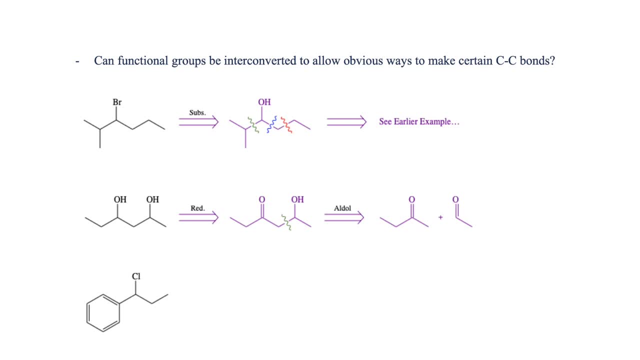 because there really aren't any good carbon-carbon bond forming reactions that result in an alkyl halide. But, similar to what I saw up above, I know that an alkyl halide is just as good as an alcohol. They're essentially the same thing. 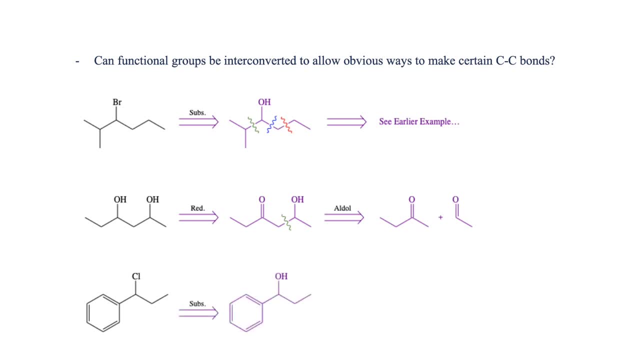 I can interconvert them through one simple little reaction, a substitution, And that means that this particular alkyl halide could have come from that alcohol of different chemistries. I mean, it's an alcohol. I could have done this and reacted, say 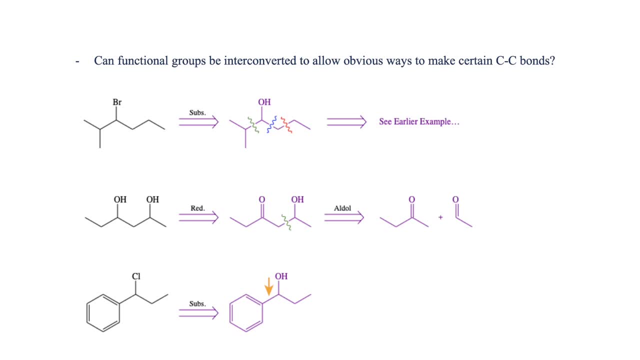 phenyl grignard with propanol right, an organometallic reaction. Or I could have taken benzaldehyde and reacted it with ethyl lithium. That would have made this bond here same idea. Let's take this a little bit in a different direction, because this alcohol is. 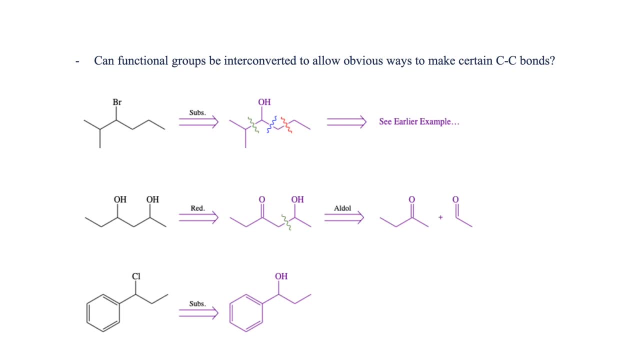 also just as good as another functionality. That alcohol is just as good as a carbonyl. I could have gotten to that alcohol via a reduction. So if I undo that, if I reoxidize it back up, I can make a carbonyl. And now what I have is a carbonyl right next door to a benzene. 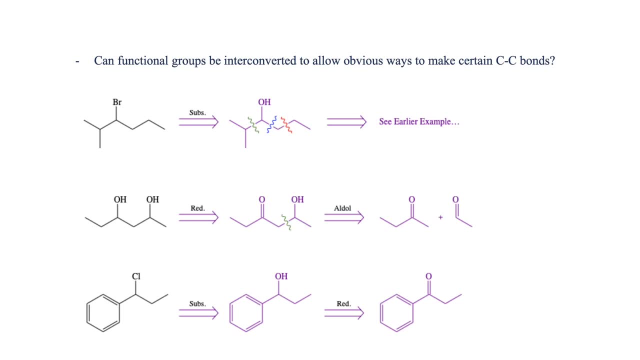 ring, And that means that I could have done what I did up above. In fact, this is the same molecule that I showed you a little bit ago. I could have made this carbon-carbon bond via Friedel-Kraas acylation, or I could have created a carbon-carbon bond here through a. 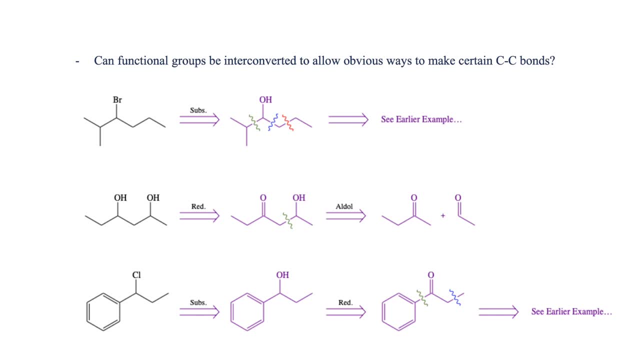 simple alkylation of acetophenone right. So this is a little bit more challenging in that there's a lot of different ways to approach this. We could have kind of unwound the original alkyl halide. We could have unwound it to an alcohol and then did some organometallic chemistry. 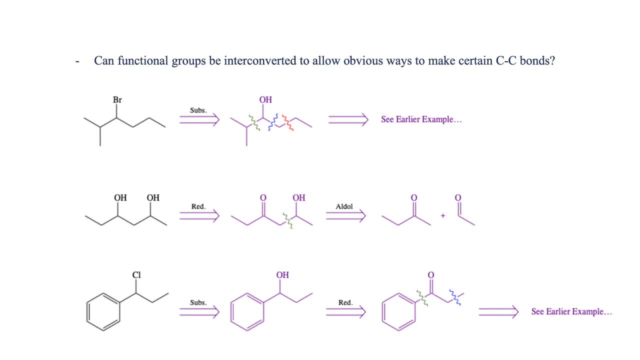 on it to make that particular molecule. Or we could have taken it one step further. before getting to the carbon-carbon bond forming reaction, We could have tweaked the oxidation state, lifting it up to a carbonyl, and that would set up, say, a Friedel-Kraas or a carbonyl. 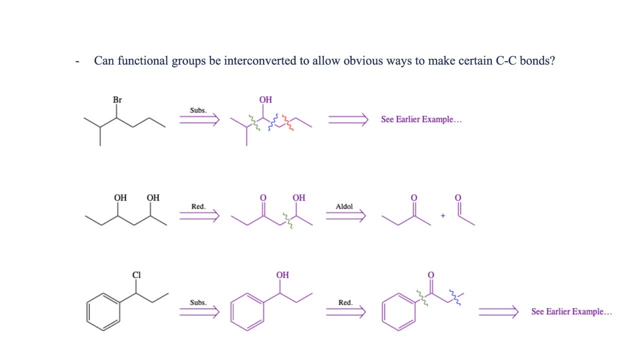 alkylation. So getting good at synthesis takes practice, And these retrosynthetic skills will really go a long way to kind of enhancing your ability to approach synthesis problems. Thinking retrosynthetically is really the way to go In the real world. there is no other option If you think about 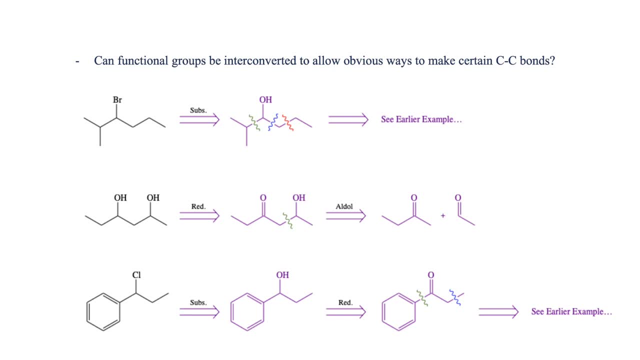 it. a lot of synthetic chemists wind up going into the pharmaceutical industry And if a new drug is discovered here we have, say, a target molecule. Hey, there's this new drug, We need to make it. We're going to ask with making it. They don't specify what to start from. You have no idea. 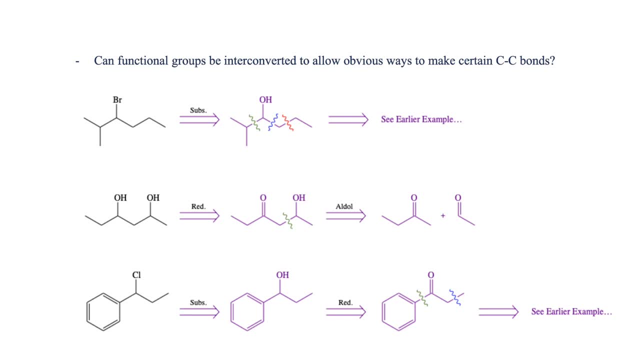 what you're going to start from. The idea is to make that molecule and that's what you know. You know what you're making. You have no idea what you're ultimately going to start from. They don't come to you and say: make this molecule, and you have to start.